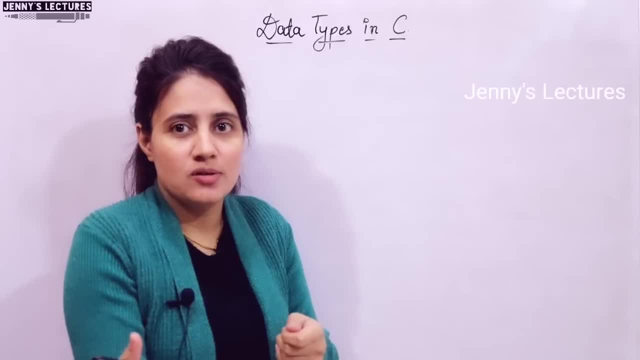 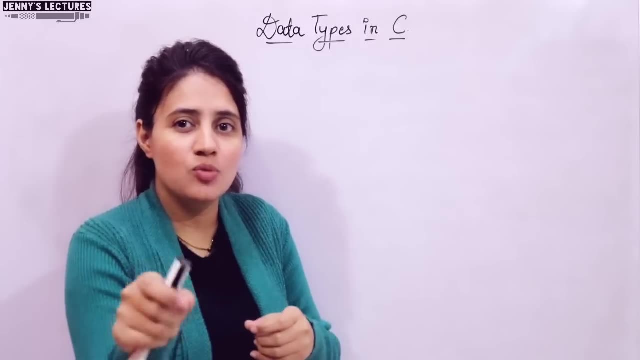 Maybe where you can put your luxury items or cash. So, according to requirements you you take those that. that space, You need that space. It's not like that in a small drawer. you will put clothes right And also you can take a one more example, like, suppose, if you want to drink, 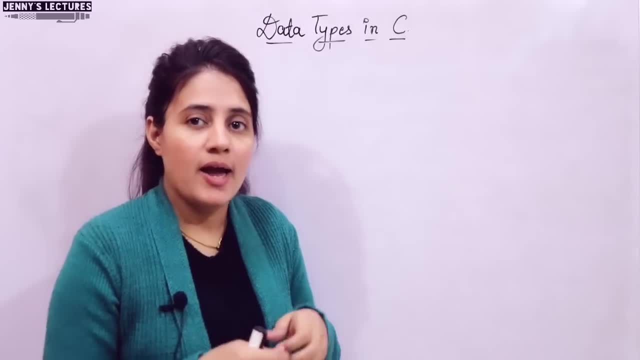 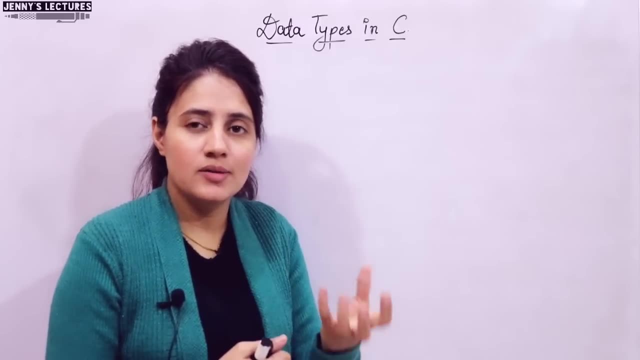 water, you will put that water, You will take glass and if you want to eat something like uh, if you want to uh eat any vegetables, then you will take what Uh, that bowl There. you will put that with that drawer. If you will have paper and清 bag, if you will have paper in the 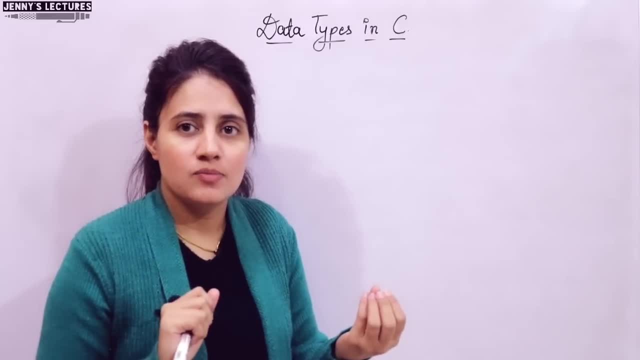 drawer. There you will put that wood if you will have paper and Wu what thaw it. The documents welcome thoughtsplinかな at that. you will come up in the description for that and they will give ChiLians and vegetable. it's not like that. you will put that vegetable in that glass. so according to requirement, 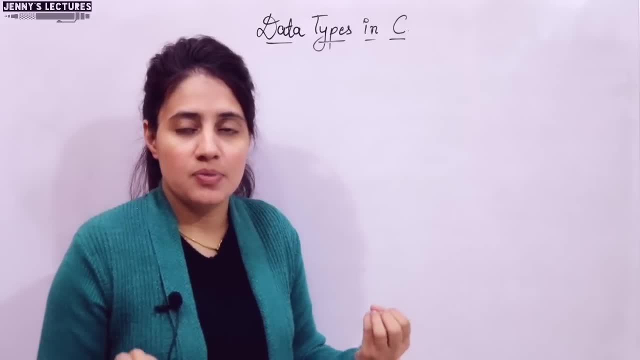 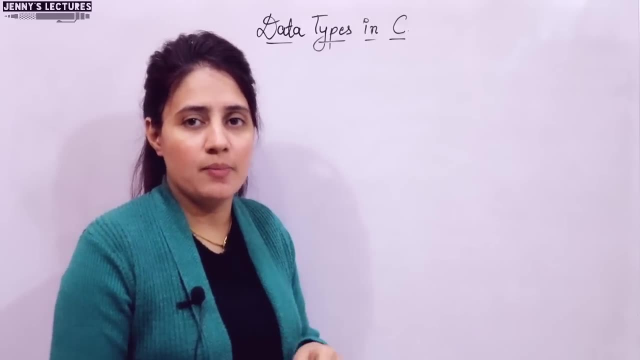 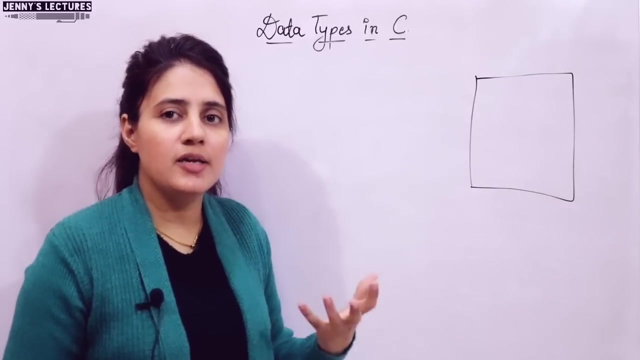 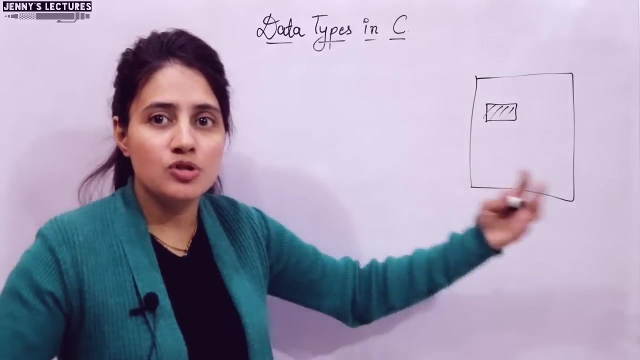 you will take those things right in computer memory also, according to our requirement, we reserve space in that memory. suppose this is computer memory, and while i'm processing, while i'm writing a program, suppose i need some space. so according to that, i will reserve some space in this memory. suppose i need more space. according to that we 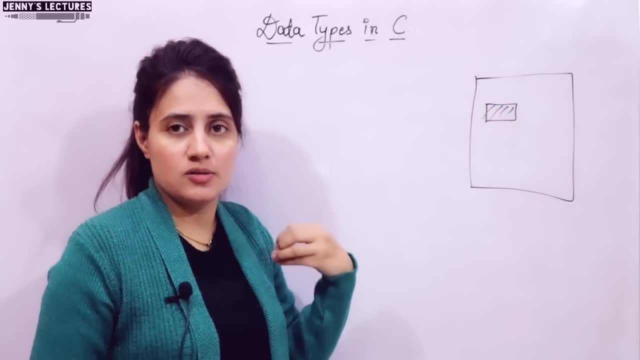 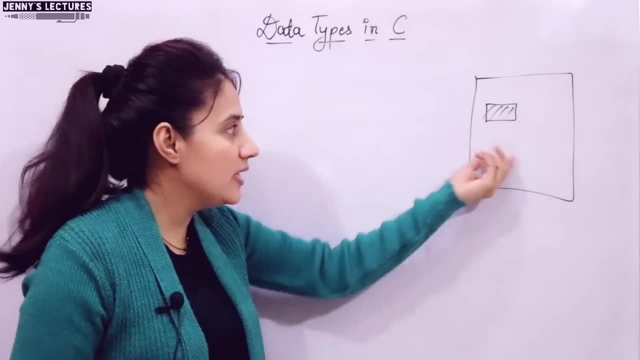 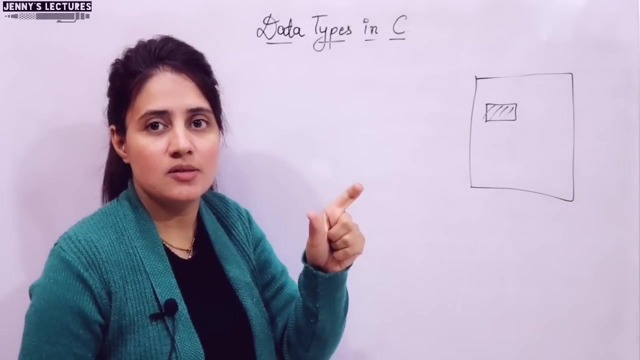 reserve, or the that computer will reserve that space for us according to our requirement, right, according to our type of requirement. now, how we specify how much space we need in memory, that is specified by data types: data types, as the name suggests. it tells you what the type of data. 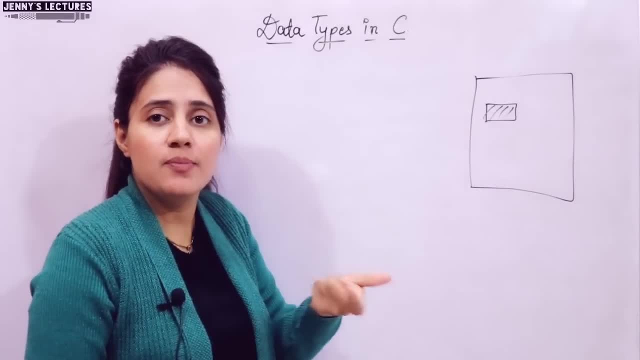 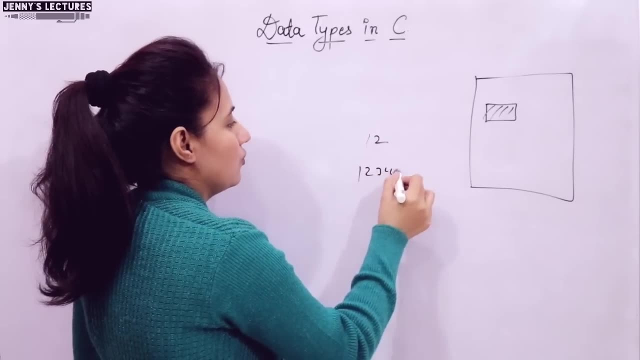 you want to store some data in memory, but which type of data you want to store? whether it's a number like 12, whether it's a number like 1, 2, 3, 4, 5, 6, a long number, or whether it's a character like a, or whether it's a string like 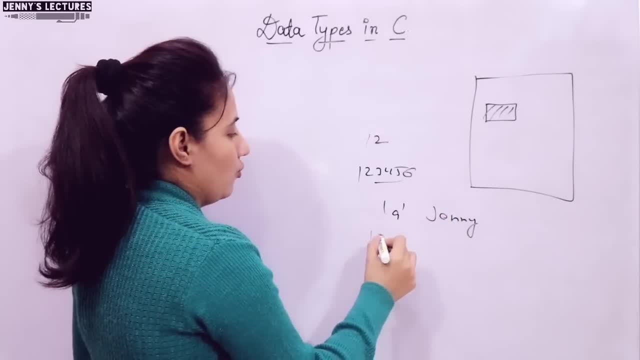 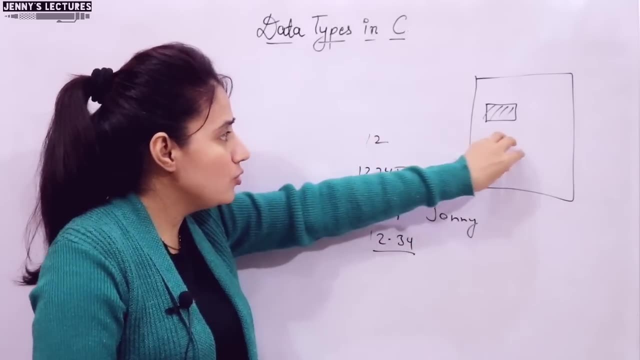 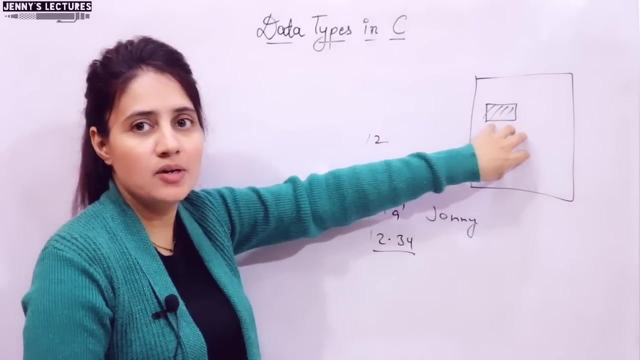 jenny, or maybe it's like one, two point three, four. maybe it's a floating point number. so which type of data you want to store here, according to that that we are going to reserve, that computer is going to reserve some memory for us so that we can use? 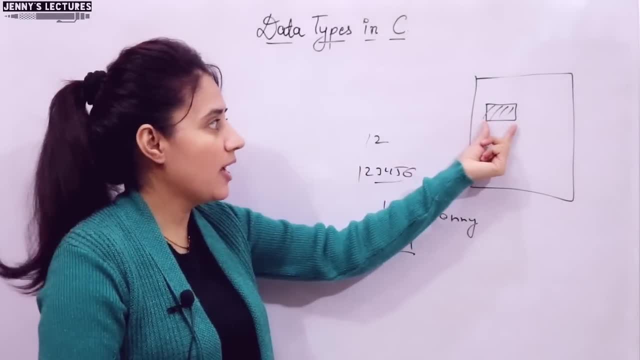 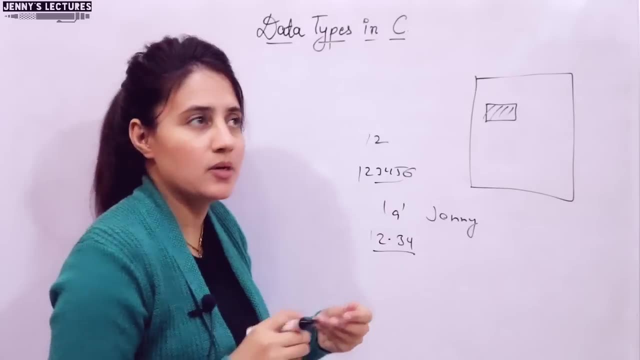 that memory, we can access that memory right. and when we name that memory, like i have told you what are variables, it's just a name given to a memory location so that we can easily access that memory, like: suppose i have given a here and suppose i have, uh, written. a is equal to 12 and 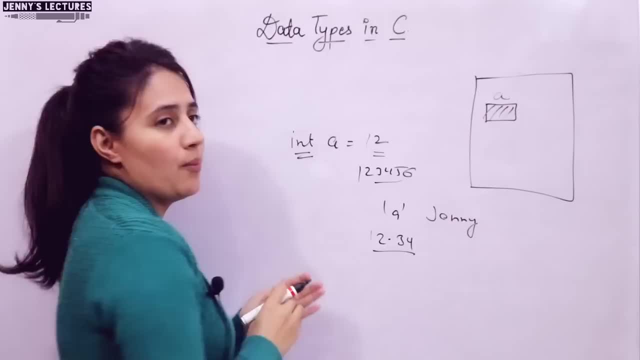 type is int, so some memory would be allocated, how many bytes, that we will discuss the size of integer, and there i'm telling you that this is a memory location and so that it can be used for various purposes, as you can see, so that when we are writing hierarchical入 and then we can use, then 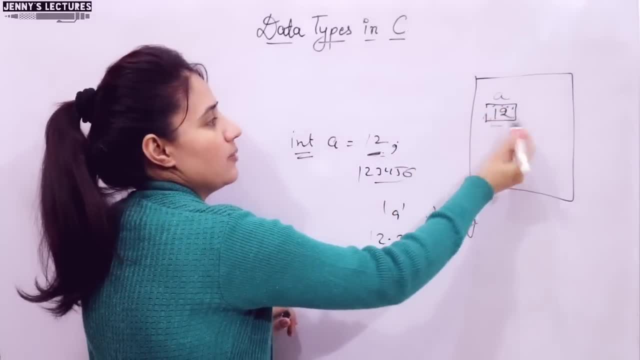 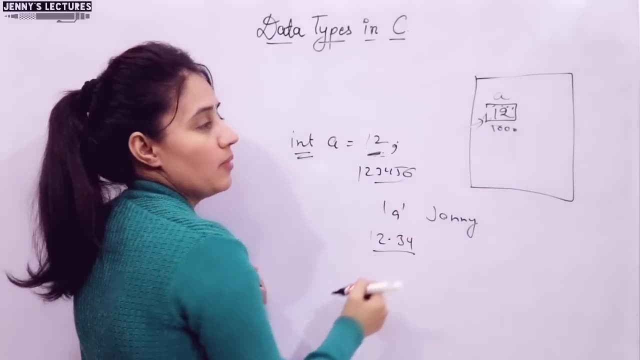 telling that you have to store 12 here. the value is 12 and some address would be there, like address is 1000, let us suppose. so this memory has been reserved for us. so if you want to access this memory, you can easily access this by calling the name, by printing: 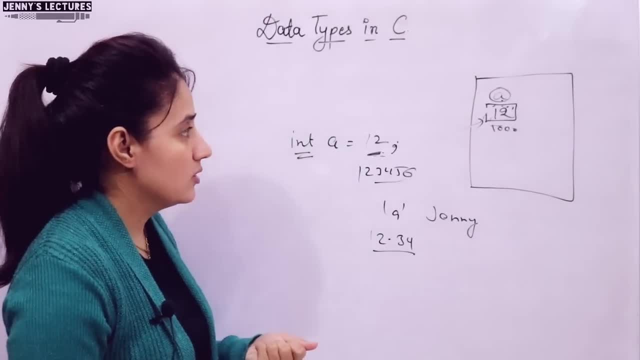 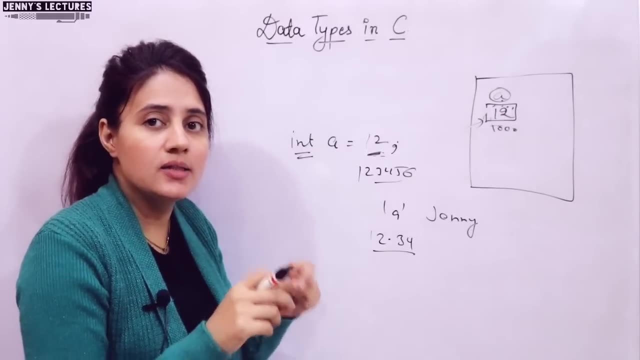 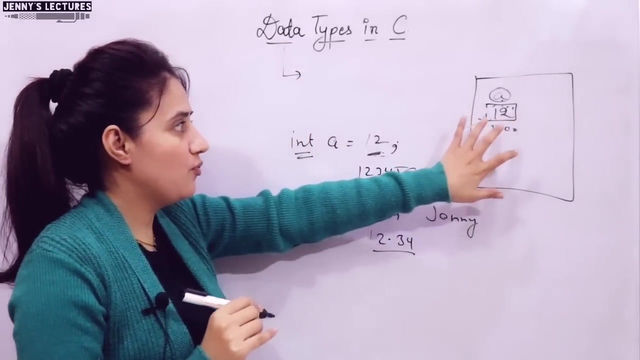 the name only right how we will print that also we will discuss. so i hope you got why we need data types in C to tell- or you can say to define- the type of data that you are going to store in a variable. so data type will tell what. first, the type of data which. 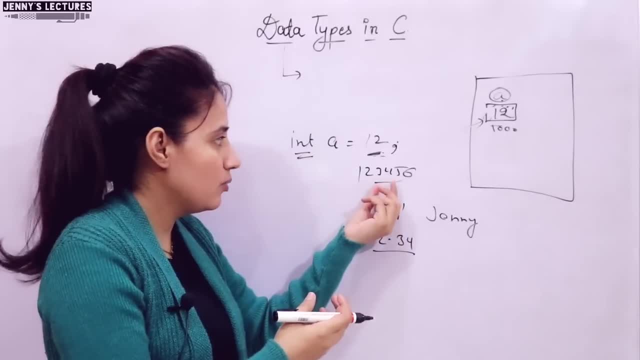 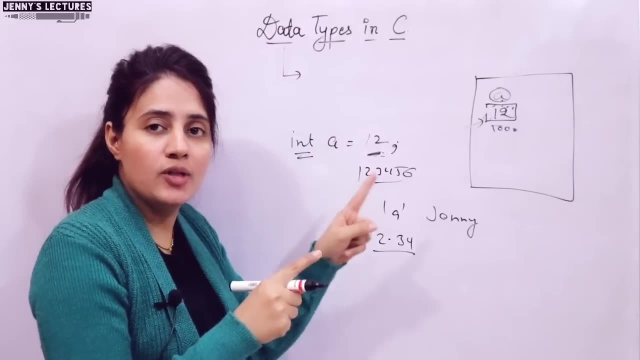 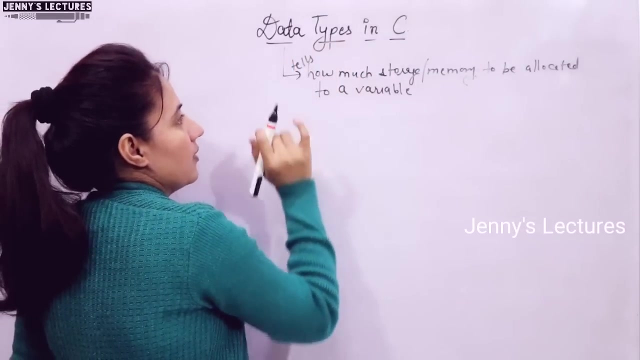 type of data you are going to store, whether it's a numerical data, floating point, integer or character or string. second thing, how much memory should be allocated to that data? see, we use data types to declare variables as well as functions. so how many types are there? how many types of data types are there? first, we have primary data types. 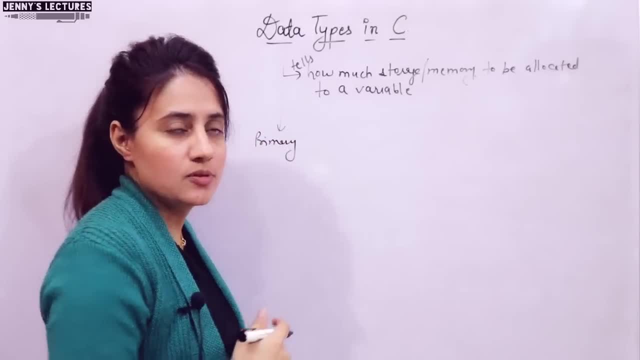 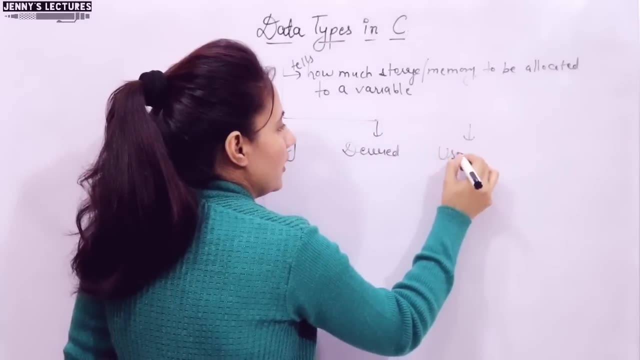 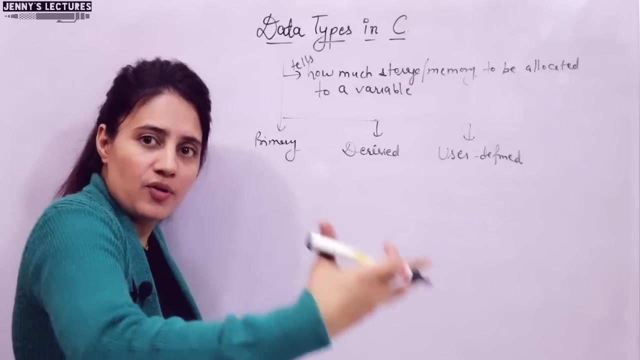 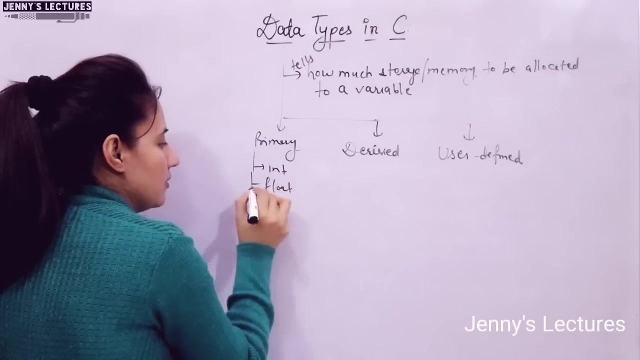 or you can say fundamental data types, basic data types. second, we have derived data types and third, we have user defined data types, see primary are also known as fundamentals or built-in data types that are predefined in that library. what comes under primary data types? int, float, char, void and somewhere it is also written that double. 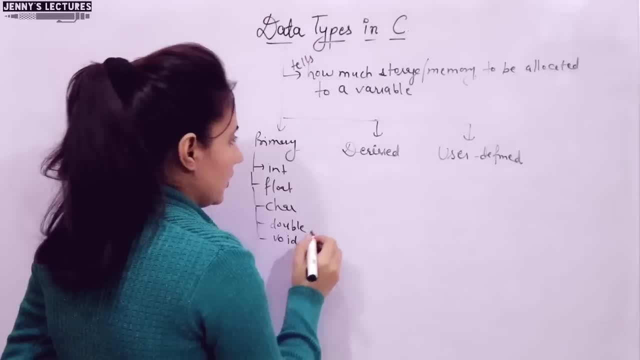 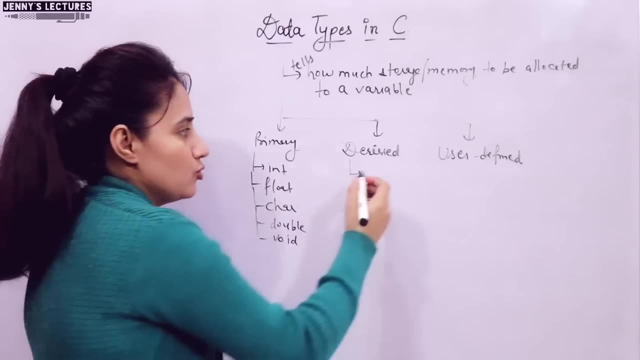 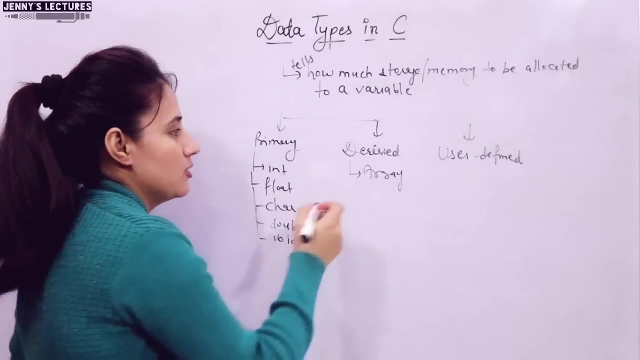 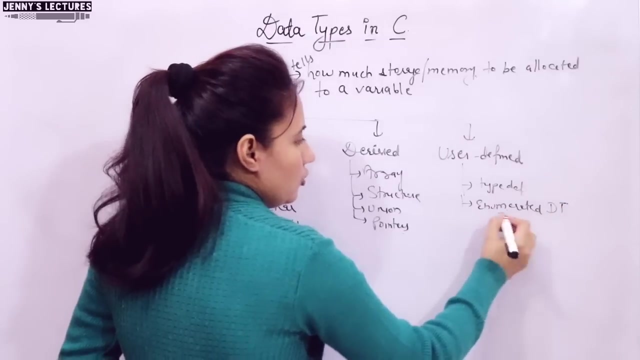 but within you can also write here double. also derived data types are: see. as the name suggests, these are derived using primary data types. so here we can say: arrays, structure, pointer, union. these are what derived data types and user defined data types are: type, def and enum. enumerated data types: see, these are separate, separate chapters in C, so we 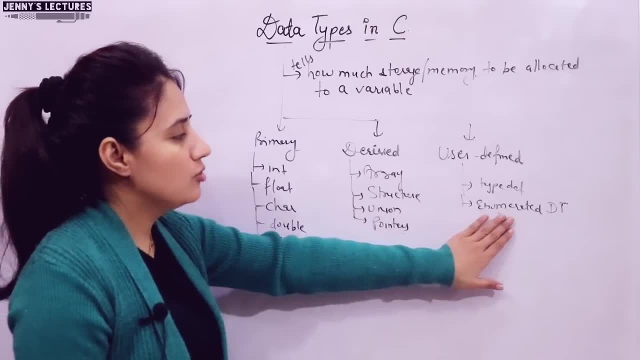 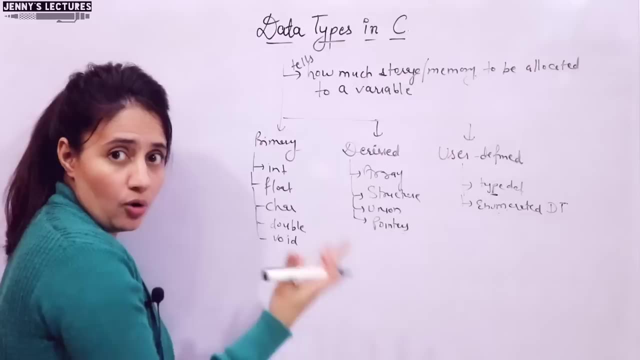 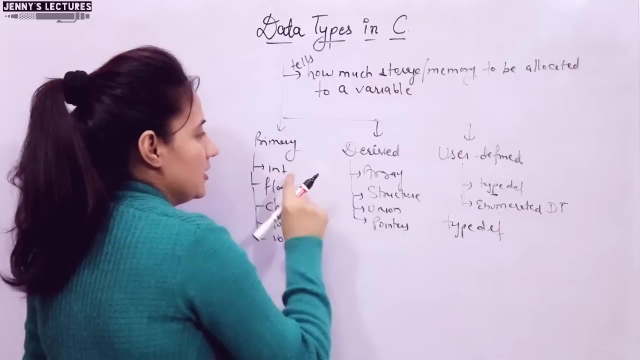 will discuss these also in separate videos and enumerated, also discuss in a separate video. type def we can discuss here. it's like you can give a name, your name, customized name, to these data types, like I am writing here, suppose type def and data type. the basic data type is int and I'm I. 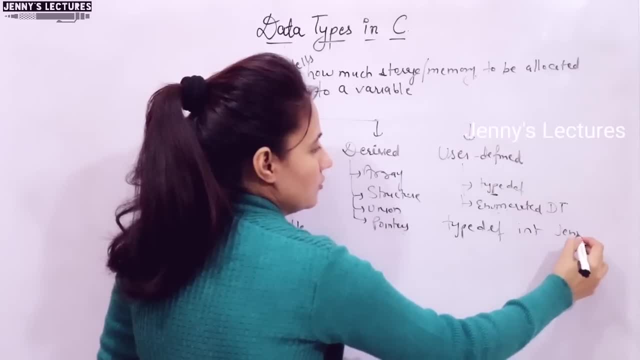 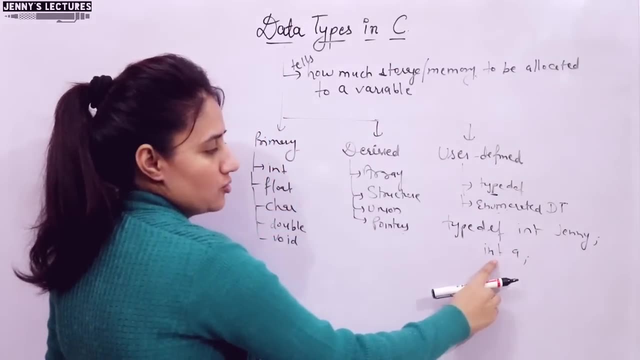 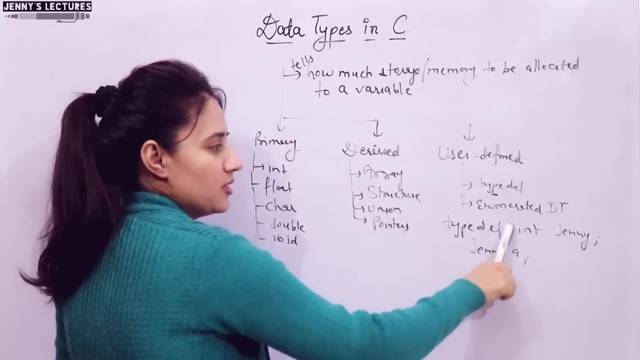 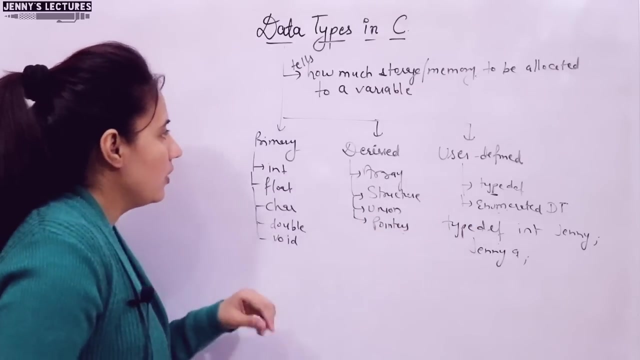 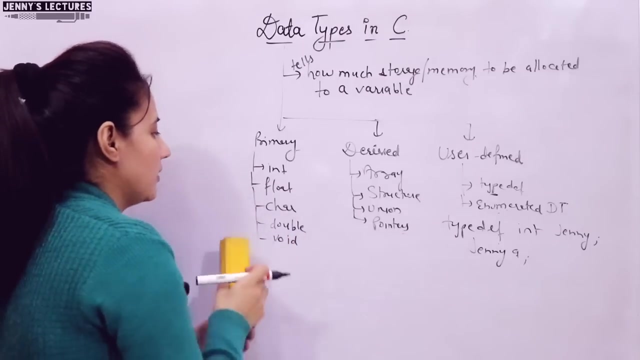 want to give a name to this data type, as, suppose, Jenny. so now when you write int a, it means you are declaring a variable of type integer. so let us write type. take a- a- a because here I've renamed it as Jenny. so this is what user defined a data type in up. we will discuss in a separate video. so in this video I am going to discuss about primary data types: what are these, why we use and the stories they need right. so first of all let us say int. int is also further categorised in short int and long int, bt, and also to do that we need black change case. 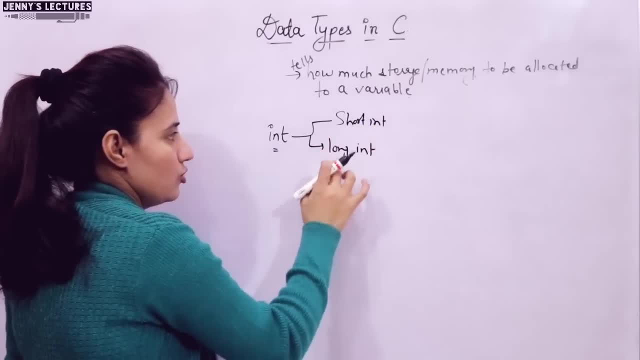 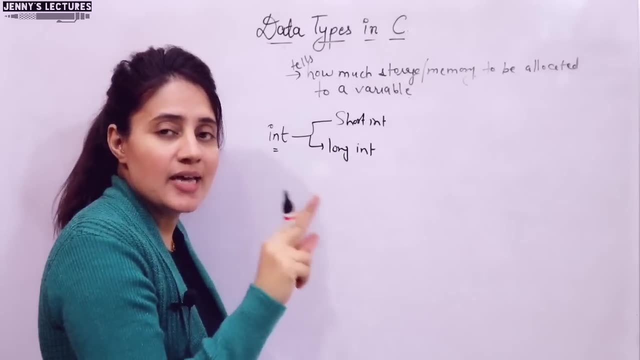 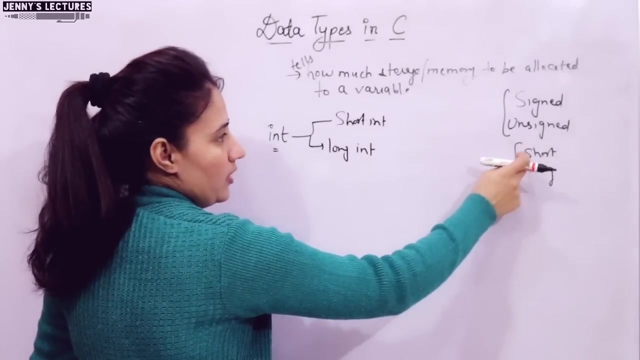 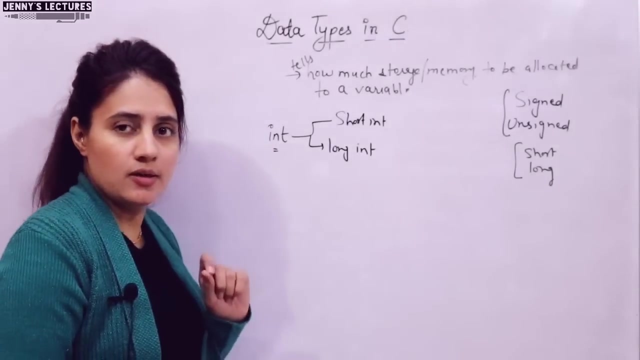 see this: short and long. these are what? size modifier, or you can say qualifiers. and further, we also have two qualifiers: sign qualifier or sign modifier, that is, unsigned and signed. so these two types of qualifiers are there: size qualifier, short and long, or you can say modifier and sign modifier, signed and unsigned. int stands for integer, you can store here. 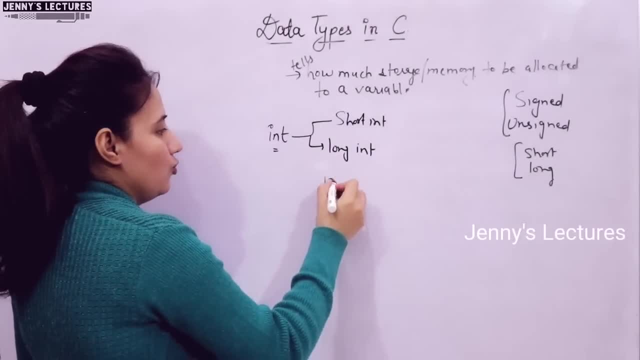 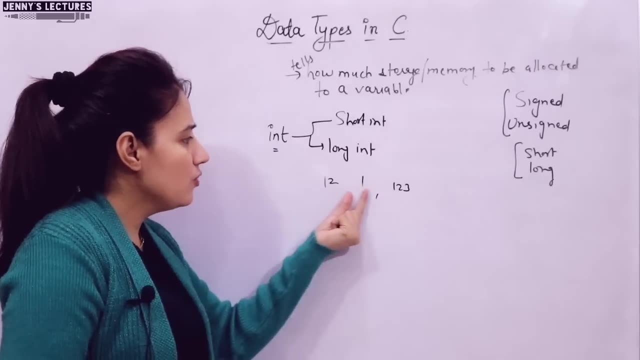 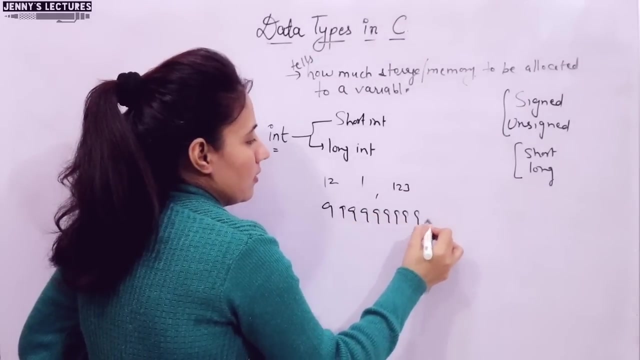 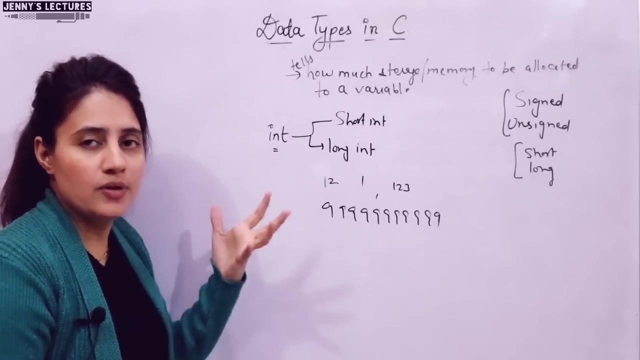 integer value. let us say 12, 1, 1, 2, 3. these are integers, value you can store here. but now, range of this integer is what suppose i want to store a number, this one, these many nines are there, can we store using int. so what is the range of integer? it depends on. 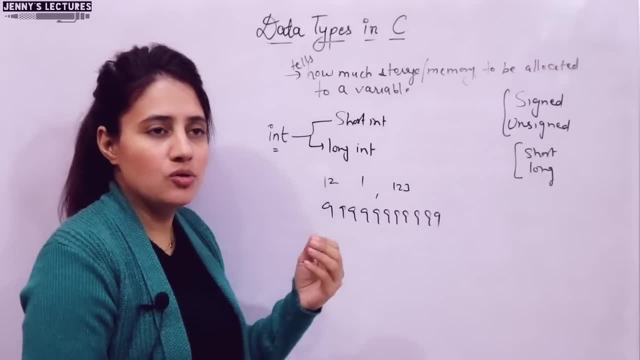 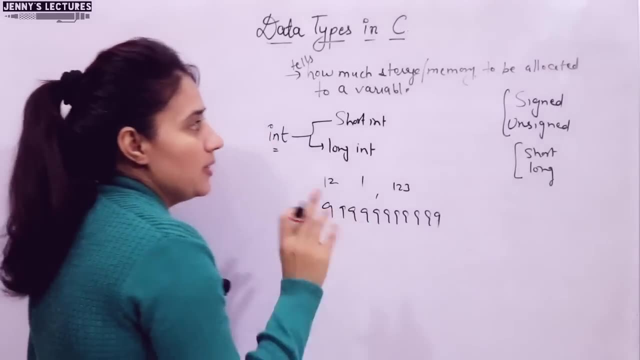 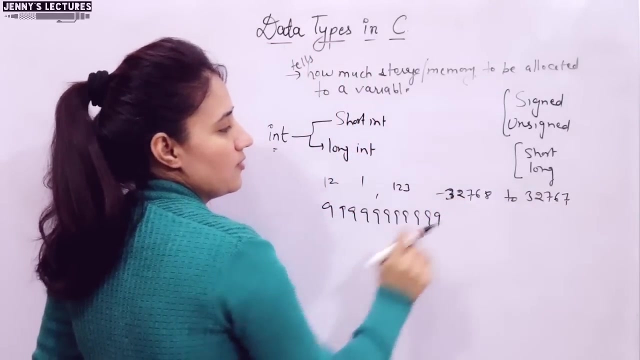 that machine you are using. you are using a 16 bit machine or 32 bit machine or 64 bit machine. that depends completely on your machine, right? so on a 16 bit machine, the range of this integer is what? minus 32768 to 32767, this is the range. and see here we are having both minus and plus. so this is what for signed integer range? is what signed integer? if you say simply int, by default, it means you are using signed integer right. signed means you can put the values negative also, positive also. but if you specify: 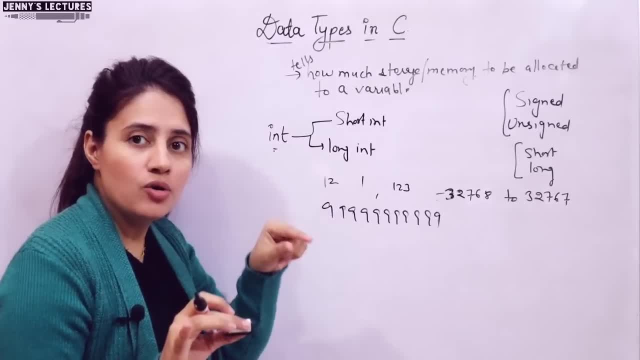 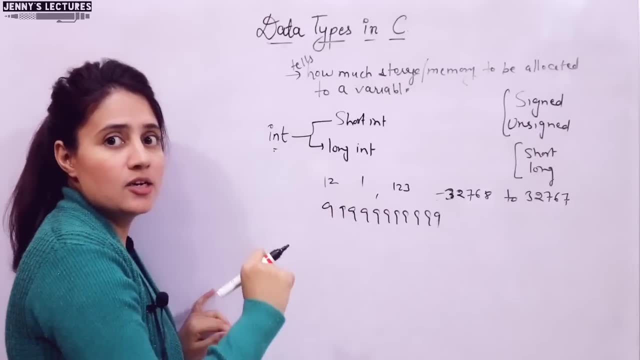 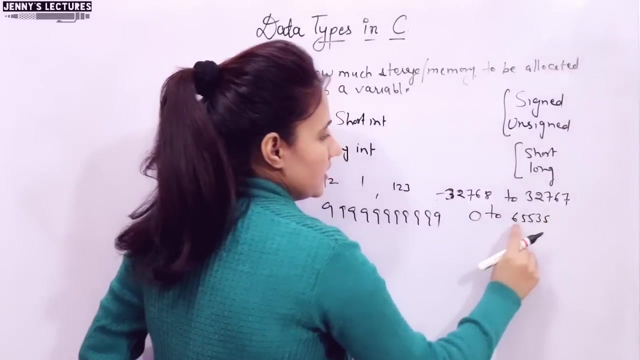 unsigned int. then you can put values, what only positive values. no sign can be there, no sign is allowed there in unsigned int. and the range of unsigned integer is what? because in unsigned we are not having negative value, so it should should be started from zero. so zero, two, six, five, five, three, five. this is for unsigned integer. this is the range that. 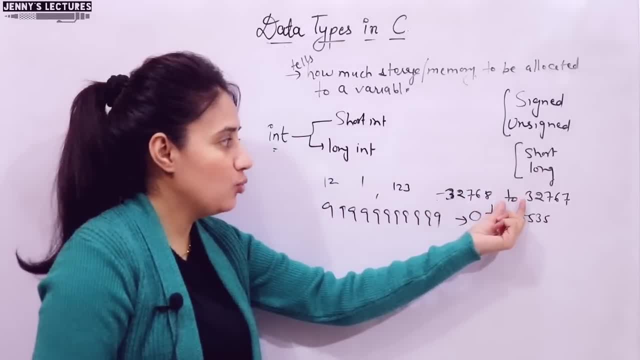 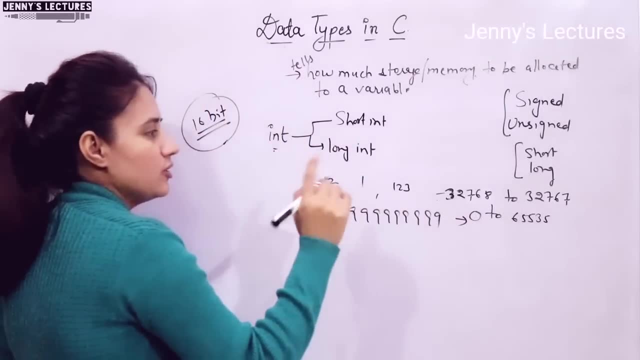 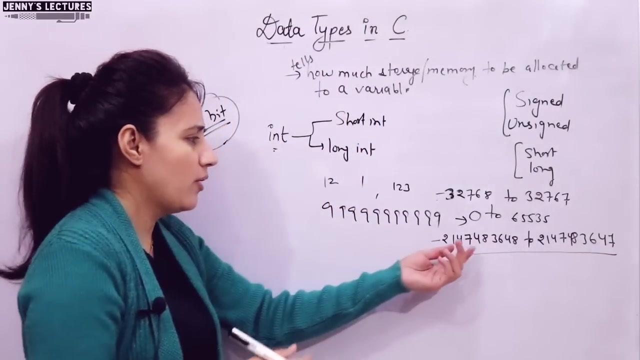 they the number you can take. you can take between these ranges only, right for a 16 bit machine. i am discussing this and, on a suppose, on a 32 bit machine, if i write the range of integer, that is, this is a range. this is the range for 32 bit machine, so you don't have to remember. 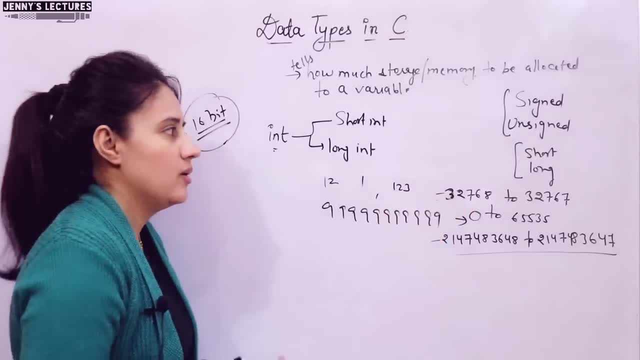 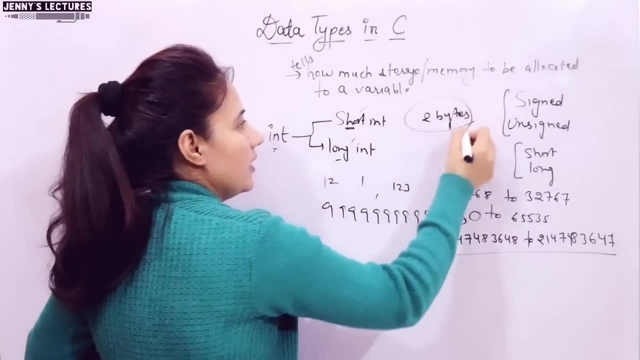 this. you just have to remember this. generally they can ask this range right and now. the memory taken by an integer is what it's? two bytes. but i'm not saying that it is a rule that you can write it in two bytes only it depends on the machine you are using. sometimes it 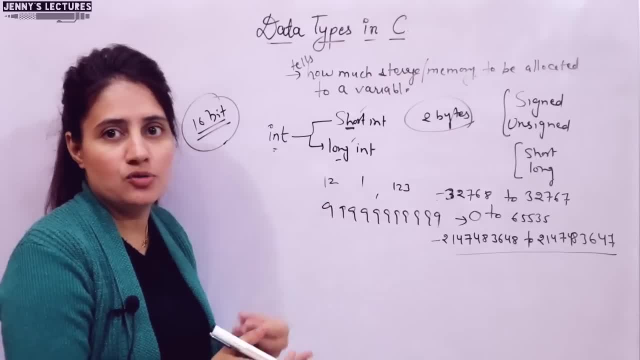 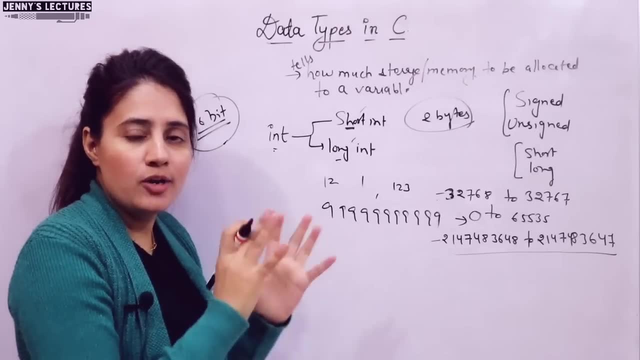 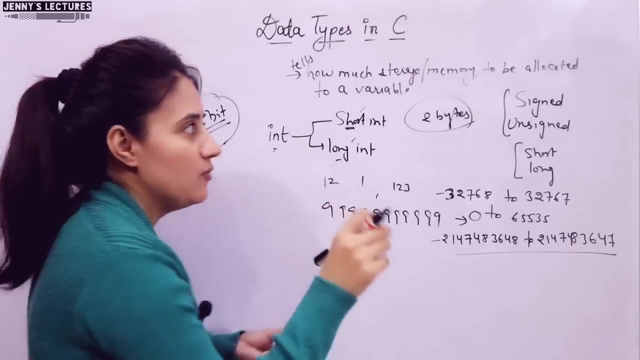 use four bytes also, and it it depends on language also. you are using c language or java language. so it's better to write a program whichever system you are using or maybe whichever language you are using. according to that, you can just write down that one statement if you want. 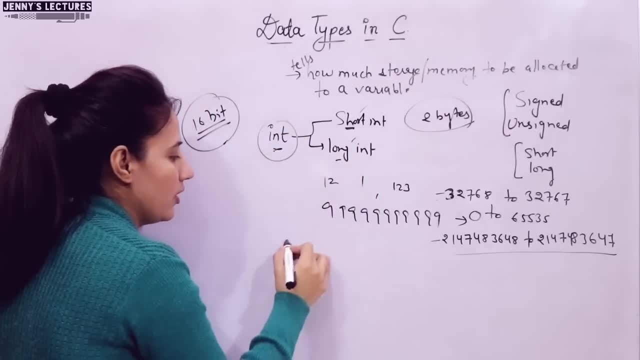 to suppose, find out that size of int. so what you can write down, just write down a simple program there. you can write down percentage f and then you can write down the number of the integer which you want to say this is equal to one, and then you can write down the. 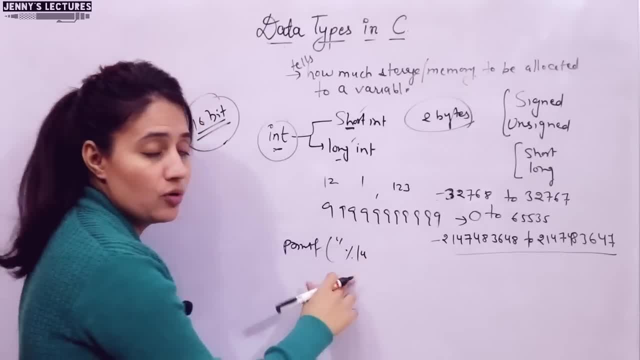 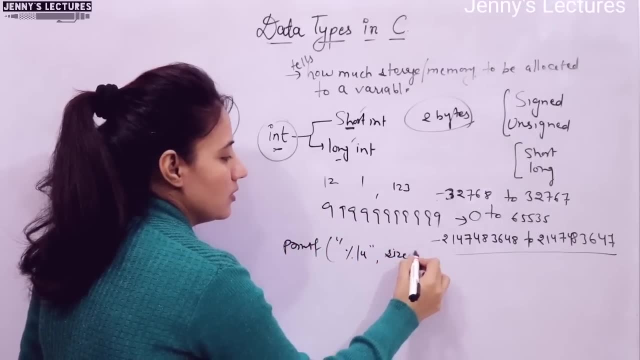 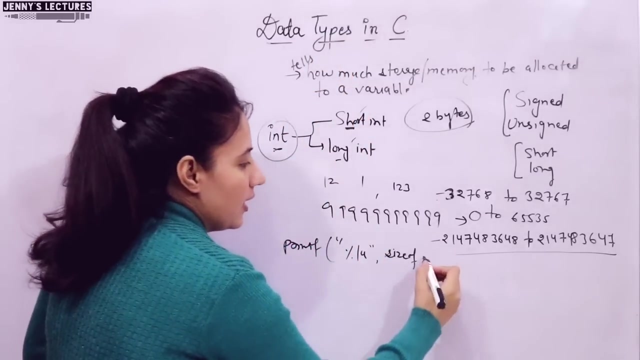 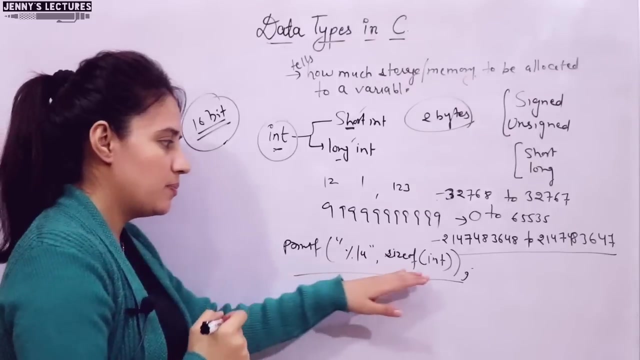 f. suppose print f percentage l? u, for it is for long integer right and here you can write simply size of size of. it is predefined function. that is in that library. we include in that header files: size of size of integer. you want to check? just write down a program and print this one like: 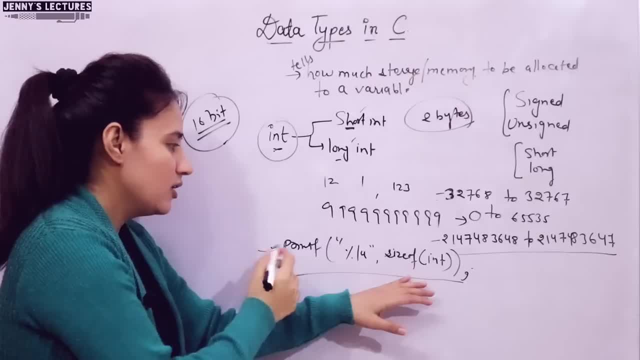 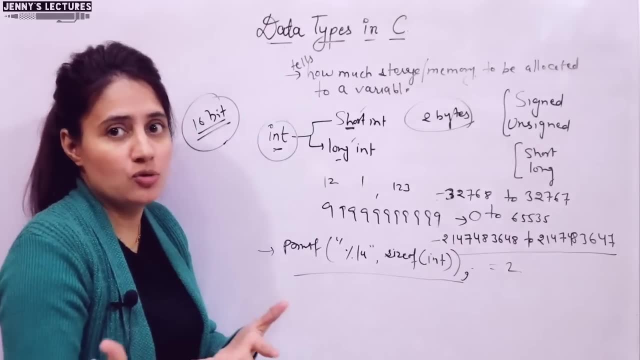 void, main and everything. obviously you have to write down. it's not like that, you just have. you just need to write down one statement only and then the size would be printed. whether it's taking two bytes or four bytes, it depends on the system you are using, the computer you are using. 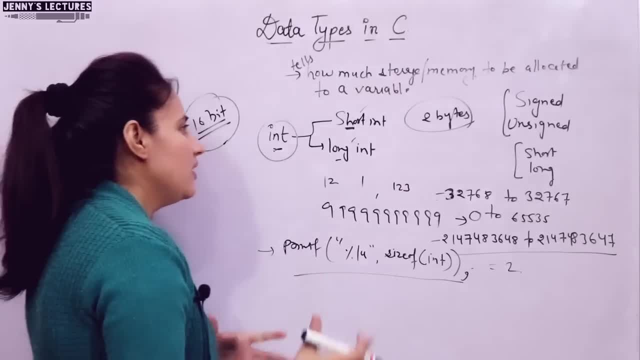 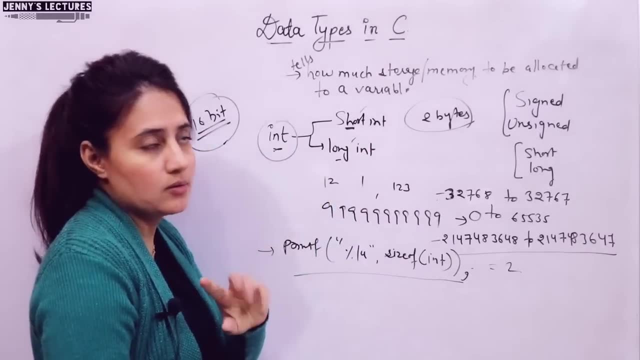 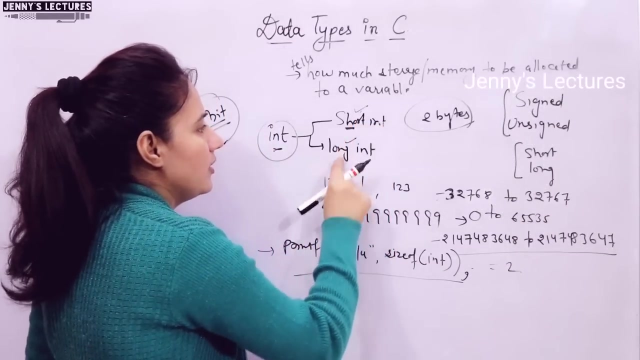 the architecture you are using. right. but generally when someone ask, or in colleges also, they teach what the integer size of integer is two bytes, but it depends, right. you need to remember this thing also now why i am writing this short and long. short int and long int. 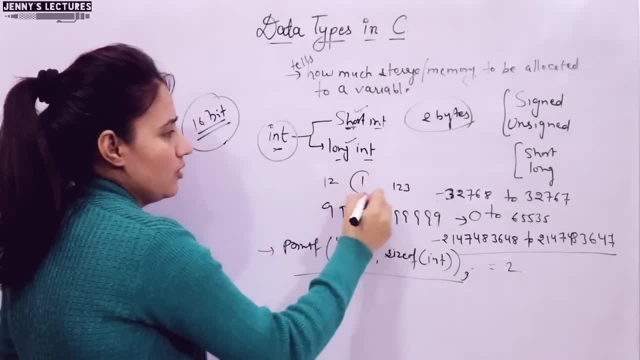 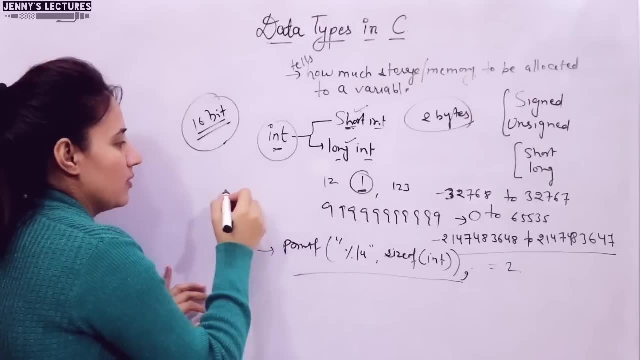 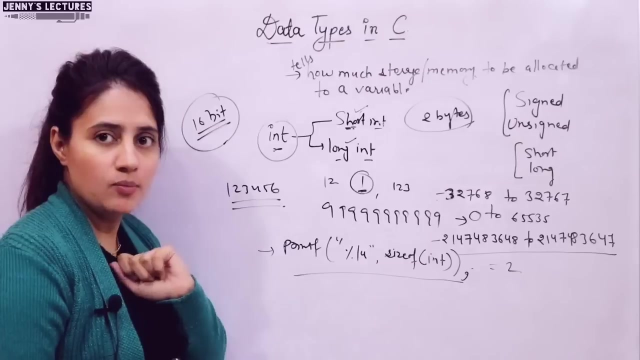 see sometimes. suppose, if you want to store single value, like one, i want to store, so i don't need much space to store one, and if i want to store like this number, then obviously i need more space than one, right, more bits than one. so, according to our requirement, we specify whether we are 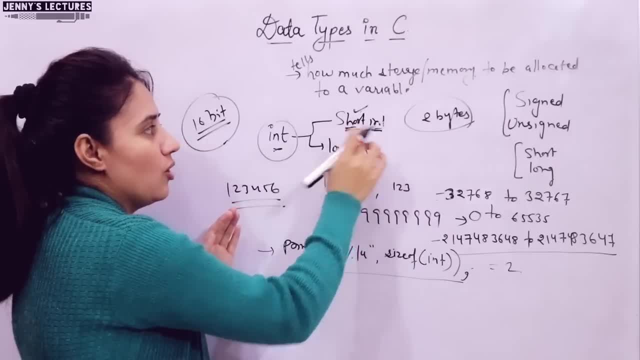 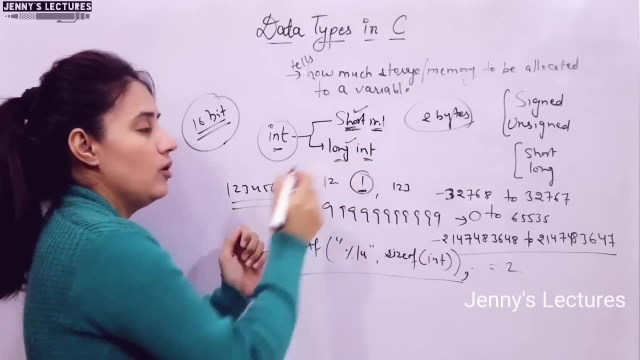 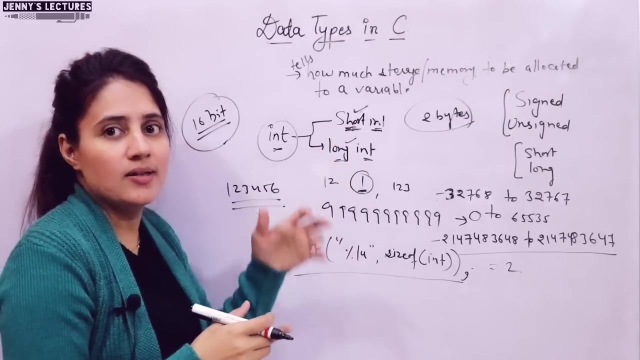 using less space, then we can use this data type short int, and if you want to store a number like that is a means, a big number, so you can use long it at the long int at that time. so, according to your requirement, you should use these specifiers rather than wasting space if you want to. suppose insert store only a number one. so for that if you take, if you use this size long end, then the size of long end would be four bytes. means long int number will take four bytes to store in memory and if you want to use long int number then you can use long int number to store. 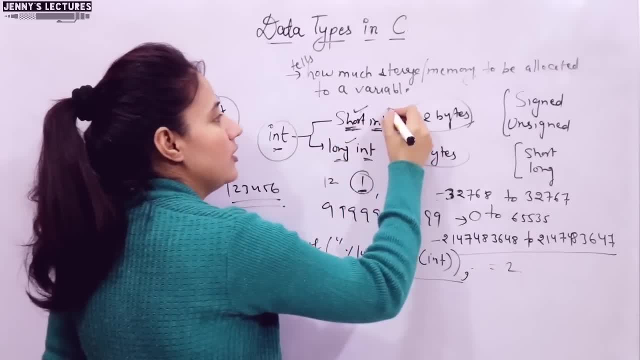 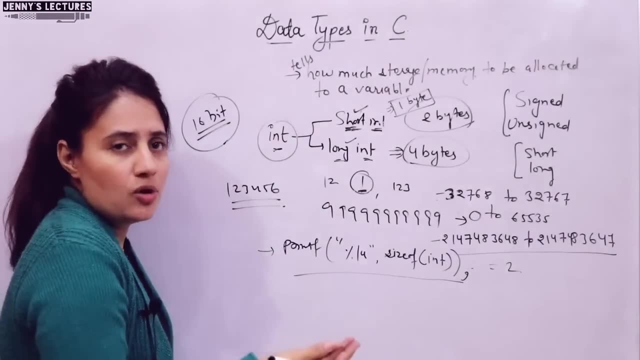 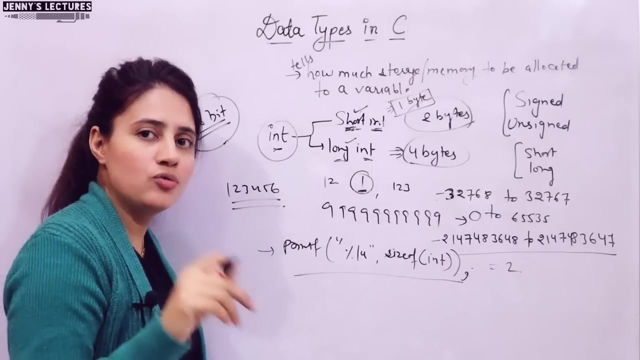 and short int. if you specify, then that number would take only one byte to store in memory. so if number is short, so use this now. why you are wasting space by using this? only? it is obviously going to slow your application only. so, according to your requirement, use this thing. that is why the 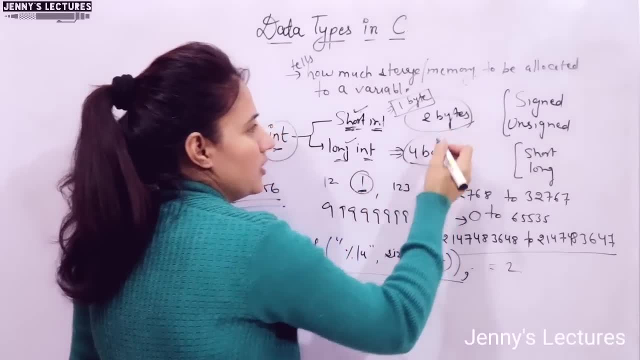 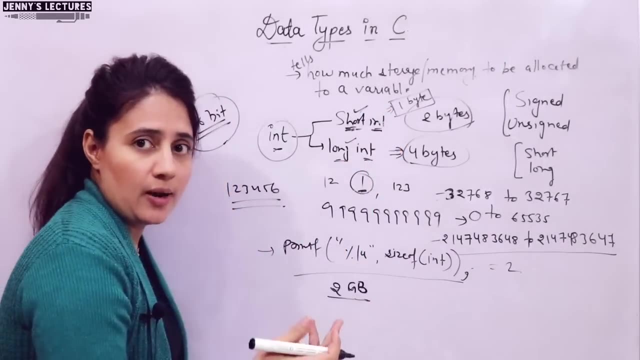 modifiers are there short and long. see here: what does this mean? suppose your ram is having ram is of two gb only, i know nowadays it is not possible to have a ram that is short and long. but if you are having a laptop with 32 gb ram, 64 gb ram ram. but just, it's a simple example. i'm taking ram of 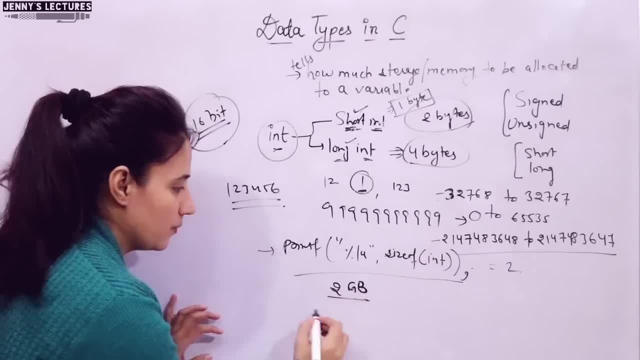 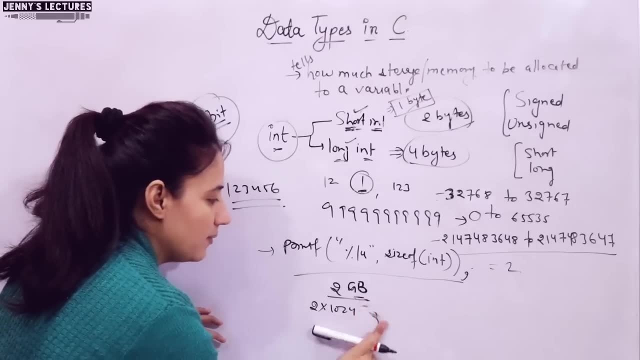 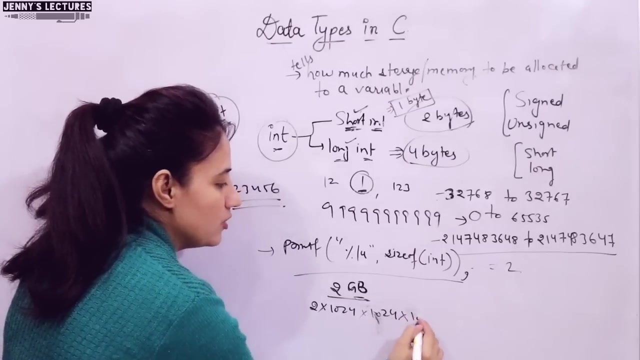 2 gb. so how many bytes, how many bits that ram can store? it's 2 into 1, 0, 24 mb and rather than mb you can write into 1, 0, 2, 4 kb and kb 1 0, 2, 4 bytes. and if you want to convert it into bits, then 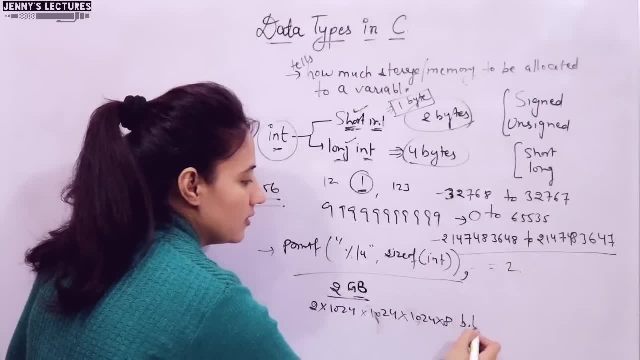 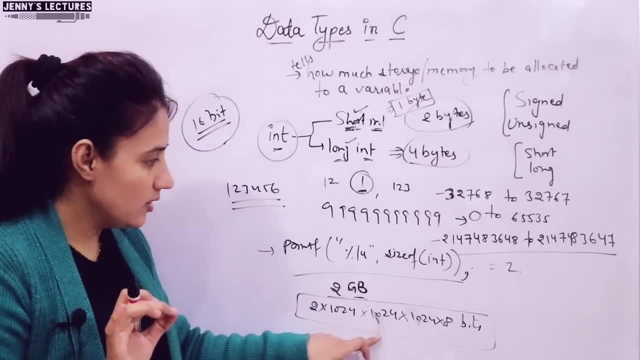 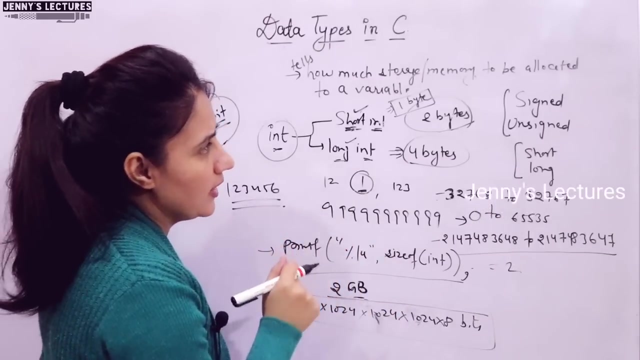 1 byte is equal to 8 bits. into 8, these many bits your ram can store, if ram is only 2 gb. so you can see how many size, how many bits we can store. right now let us discuss. this is about integer. now let us discuss about character. but before that, just want to give you some example. 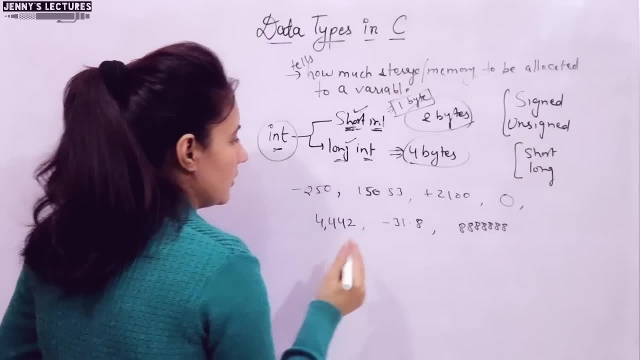 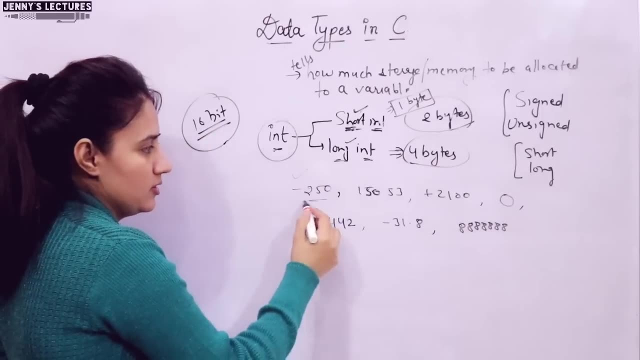 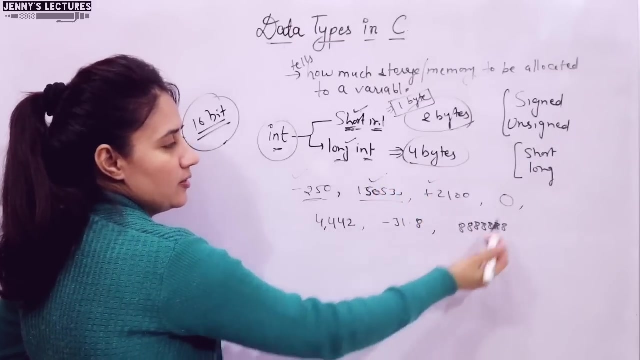 of valid integer and invalid integer: see. so see, this is what i am discussing, it in the context of 16 bit machine. so this is what valid. this is signed integer. this is also valid. there is no space, it is just 53. this one is also valid. this one is also valid, but this is invalid because 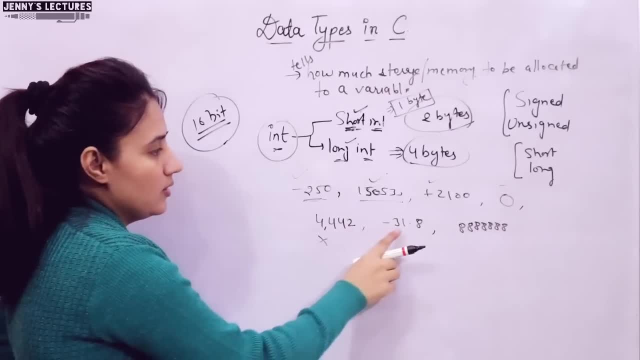 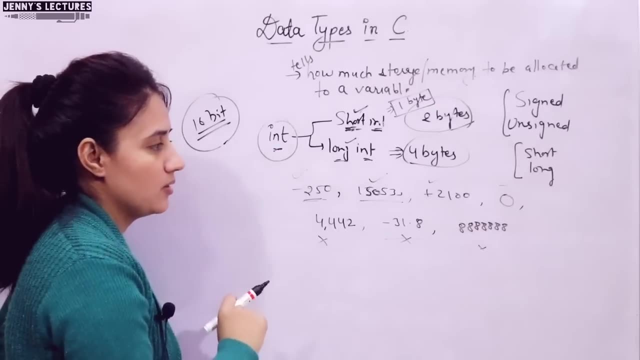 here i am writing comma. that is not allowed, right? this one is also invalid because this is decimal. this is invalid because it is out of range for a 16 bit machine. for integer and how you can print this int: you just have to use the format specifier. how you can print integer value. 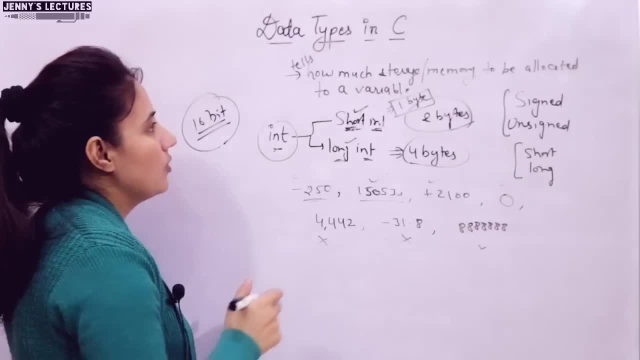 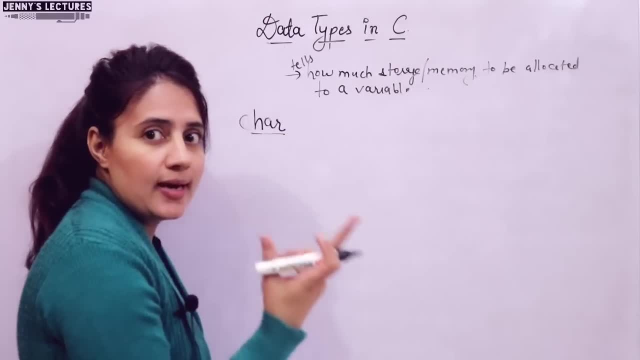 using percentage d right now. using percentage d right now about character. so it is going to store a about character. so it is going to store a about character. so it is going to store a single character, single character, single character, right, and how we will define that right and how we will define that. 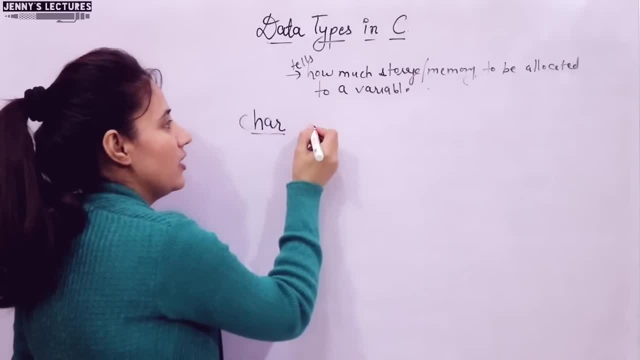 right and how we will define that character type of variable. you will use character type of variable. you will use character type of variable. you will use this keyword care and just write down the this keyword care and just write down the this keyword care and just write down the name of that variable. suppose i am. 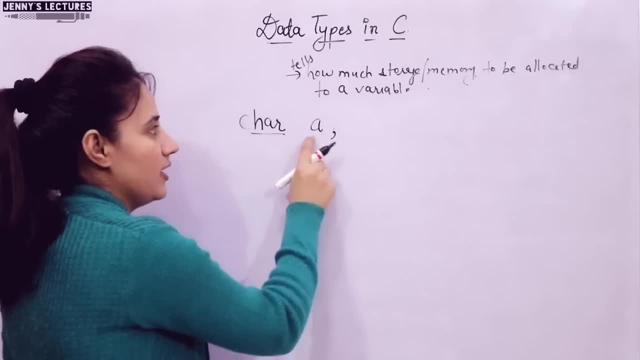 name of that variable. suppose i am name of that variable. suppose i am writing here a. that's it. this a is having writing here a. that's it. this a is having writing here a. that's it. this a is having value that is of character type and the. 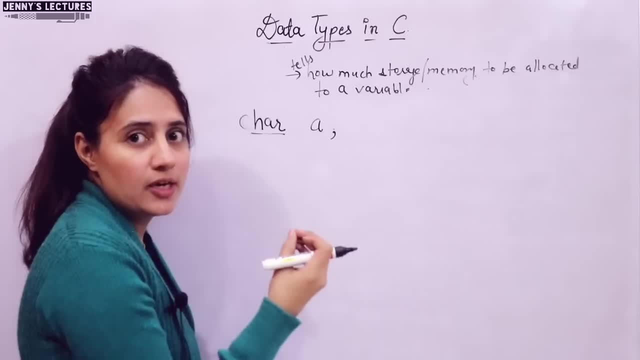 value that is of character type and the value that is of character type and the memory size it will take memory size. it will take memory size. it will take how many memory, how many bits it will. how many memory. how many bits it will. how many memory, how many bits it will take in internal storage. if you want to. 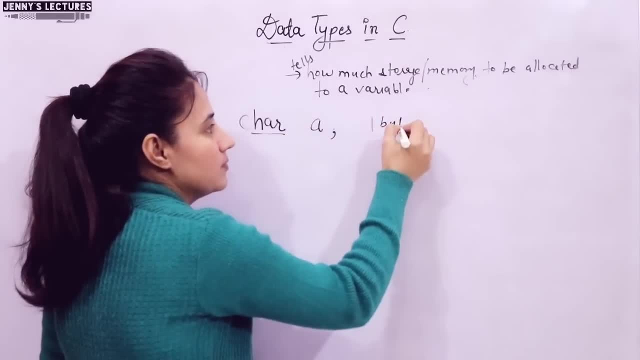 take in internal storage. if you want to take in internal storage. if you want to store a character type of variable, store a character type of variable. store a character type of variable. only one byte, or you can say eight bits. only one byte or you can say eight bits. 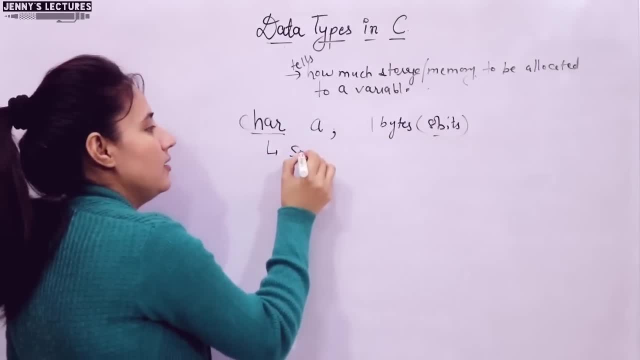 only one byte. or you can say eight bits. one byte is equal to eight bit right. one byte is equal to eight bit right. one byte is equal to eight bit right. character can be signed. character can be signed. character can be signed and unsigned, but both will take how many? and unsigned, but both will take. how many? and unsigned, but both will take how many space? one byte only, both signed and space. one byte only, both signed and space. one byte only, both signed and unsigned. by default. if i write, carry it unsigned by default. if i write, carry it. 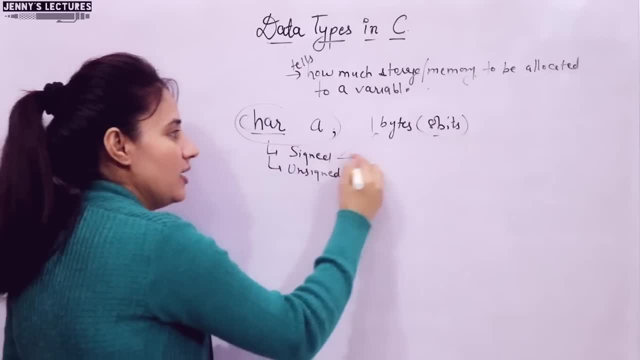 unsigned by default. if i write carry, it means means, means it is signed character and the range of it is signed character and the range of it is signed character and the range of signed character would be signed character would be signed character would be plus 1 to 8 to 1 to. 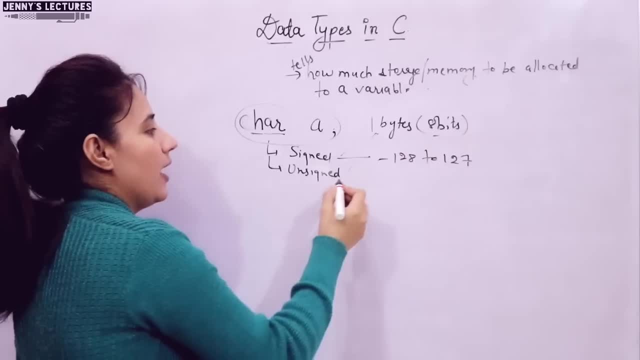 plus 1 to 8 to 1 to plus 1 to 8 to 1 to sorry. minus 1 to 8 to plus 1 to 7. sorry, minus 1 to 8 to plus 1 to 7. sorry, minus 1 to 8 to plus 1 to 7. and for unsigned it ranges from 0 to. 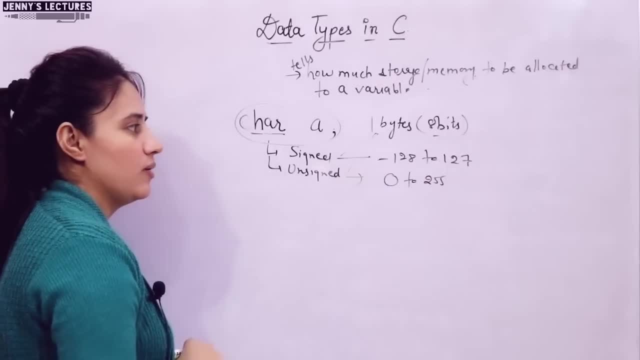 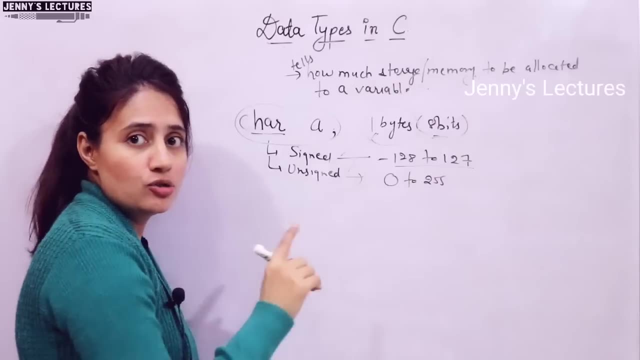 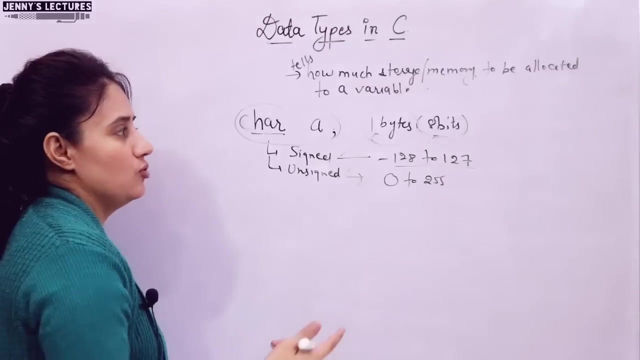 and for unsigned it ranges from 0 to 255, because here it is unsigned, so no negative value can be there. see why this range is this one and why the range of integer was this one. because using one byte, using eight bits, we cannot store a number greater than 127 and less than minus 128. same with integers: you cannot store. 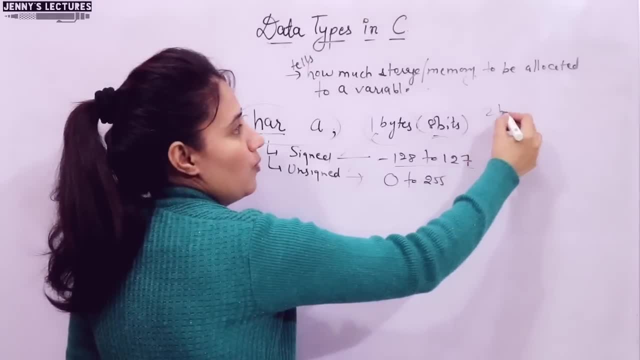 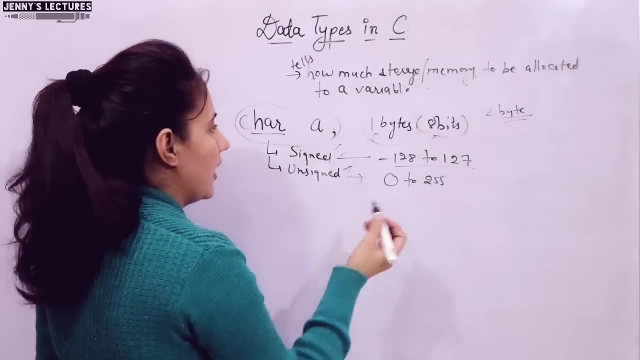 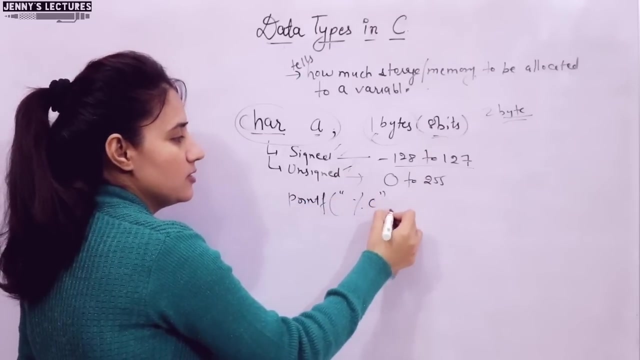 a number greater than that range using that two byte of space, because integer will take two byte. it depends actually upon upon that system we are using right and the format specifier we use for printing care is what percentage c suppose in a program. i am writing printf percentage c and if 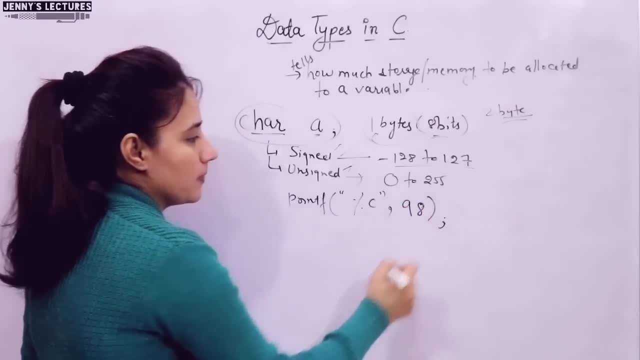 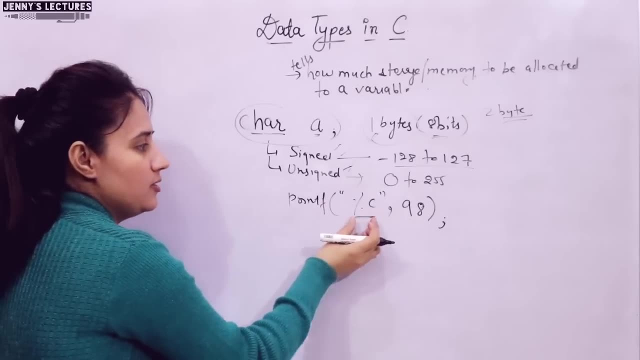 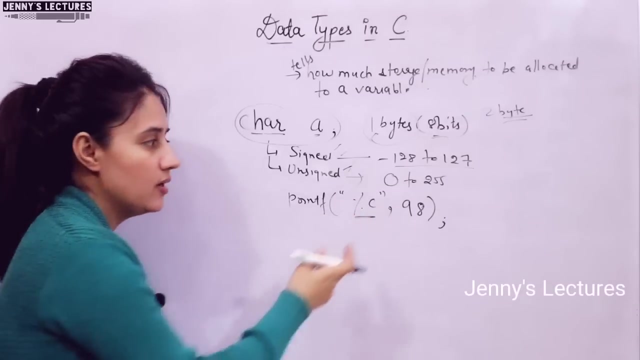 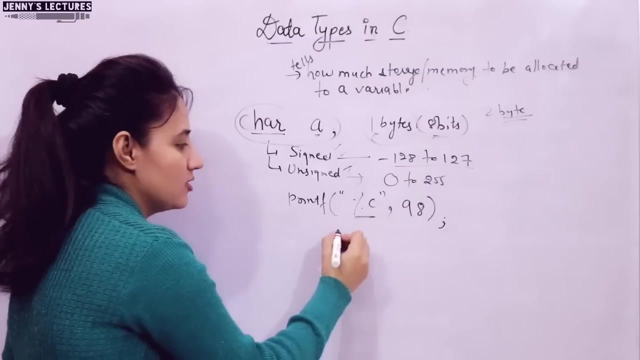 suppose i am printing here value 98, then what should be the output percentage? c means character should be output, right. it means after that this comma, the first number. it will print what character value. but here we have 98, so you will say that 98 would be printed. no sky value. this is sky value. for which character small b. 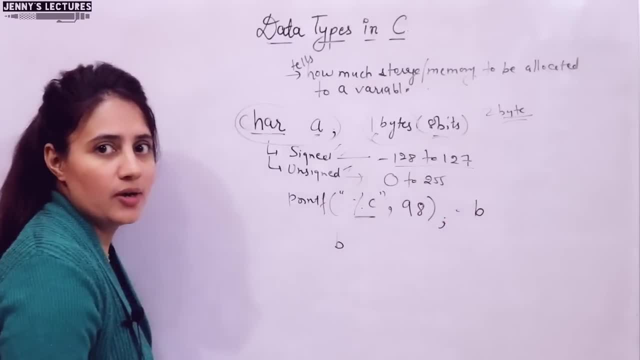 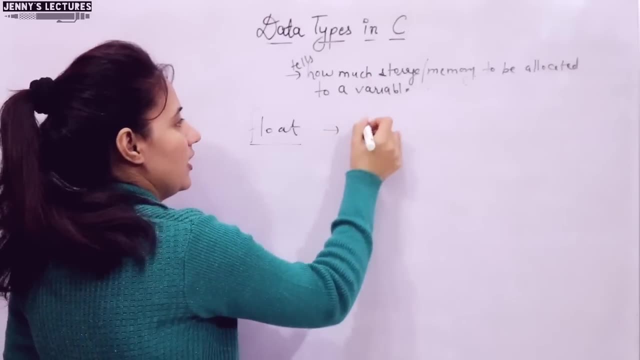 so character b would be printed. the output would be b here. so now next is float. it is used to store decimal points, decimal values, fractional values and the memory size. it will take as four bytes. the range of this float is this one minus 3.4 e. 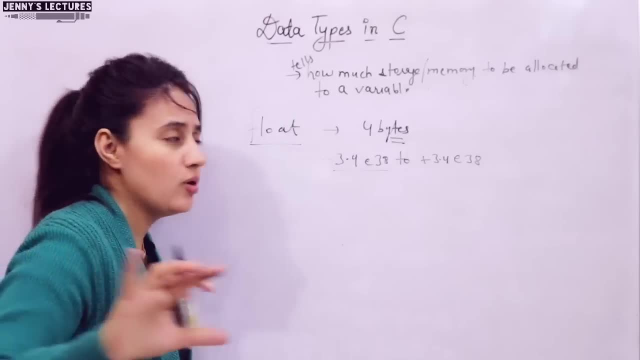 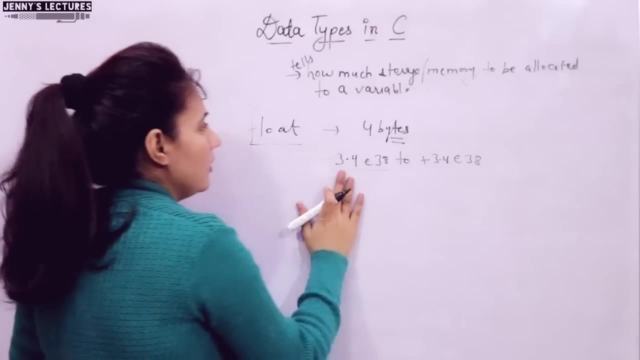 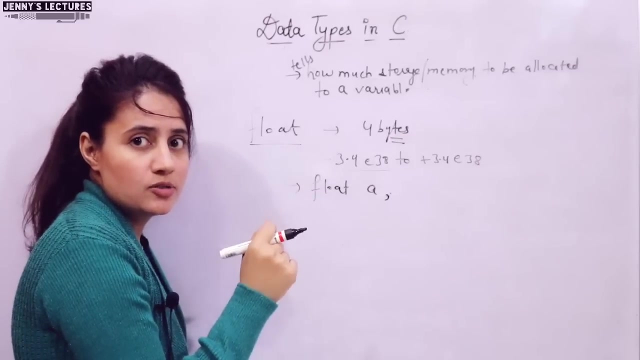 38 is e means i'm writing this number because it is a long number, so i'm writing this number in form of exponent form. this is mentissa. this is exponential form. right now. float is how we declare this variable float, float a. we can also say it real numbers, decimal numbers or floating point number. 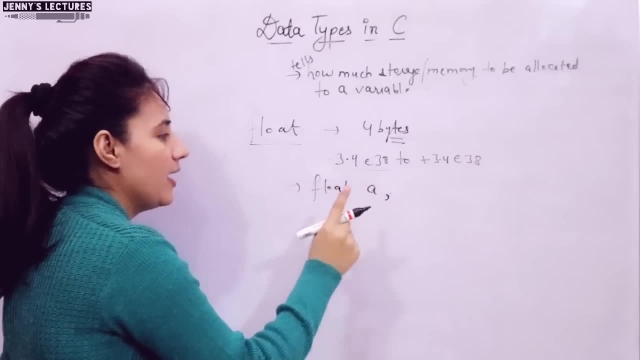 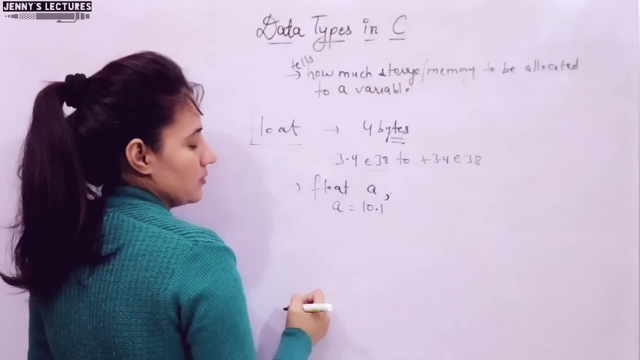 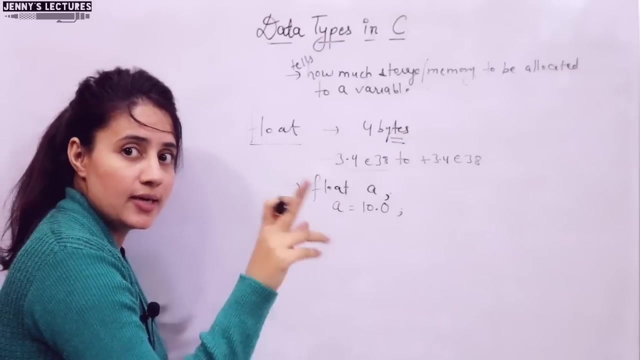 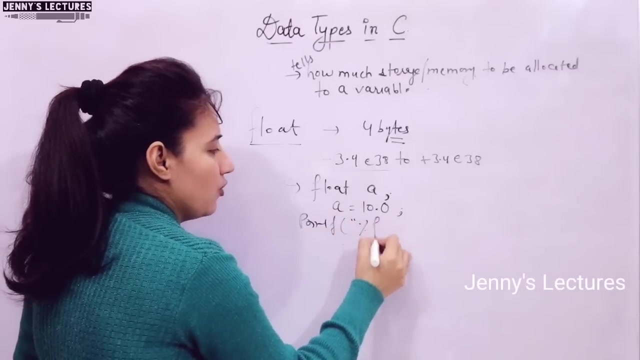 right. float a means the value of a should be floating point number and suppose value of a. I am initializing like 10.1, right, or you can initialize 10.0. also, it is not equal to 10, 10 is integer, 10.1, 10.0 is float. so if you will print this a the format. 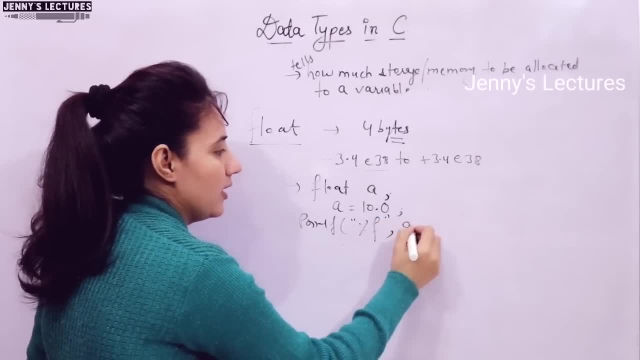 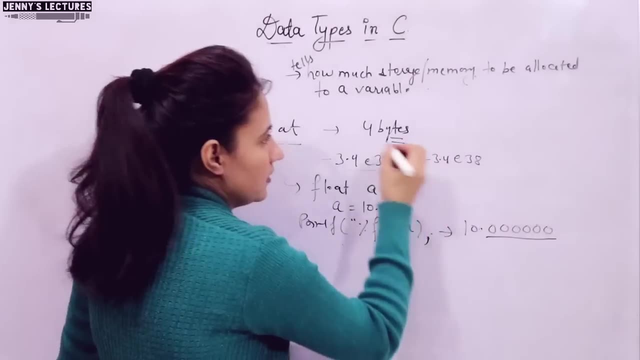 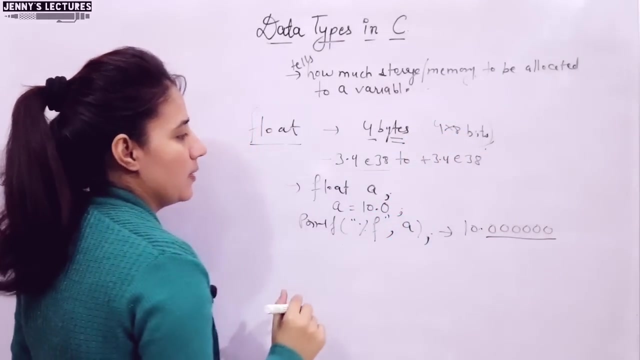 specify you will use for float is percentage f and a, then what should be the output? 10 point. the float will take 6 digit of precision is in this size in 4 bytes. 4 bytes means 4 into 8 bits. in these bits we can store up to 6 digit precision. number right and 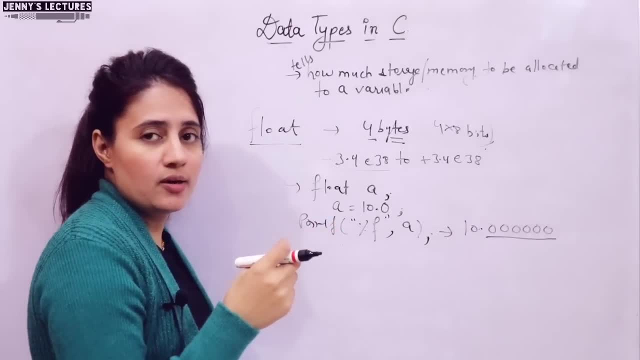 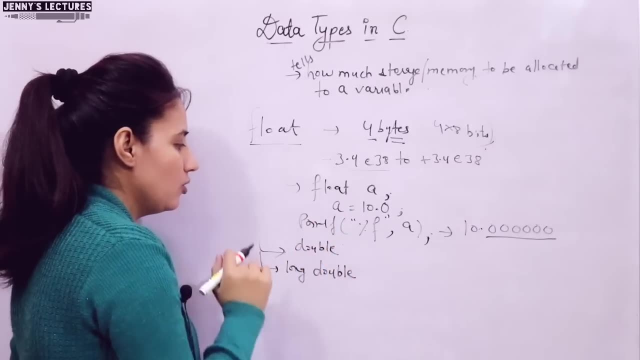 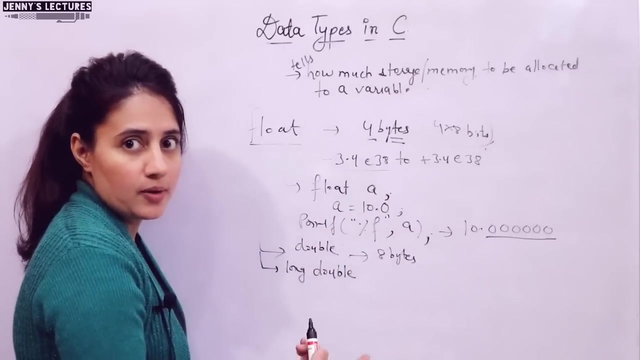 float is also having Classes or you can say it is of type double and long double. these are, you can say, 3 classes of a float, type of variable float: double, long, double. now it is taking 4 bytes. double will take 8 bytes to store a number. if a number is long, double, sorry double- then it 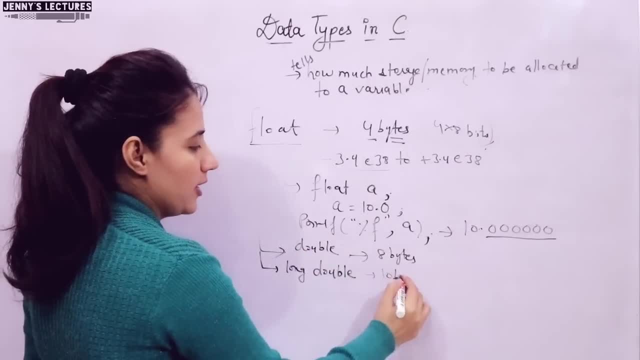 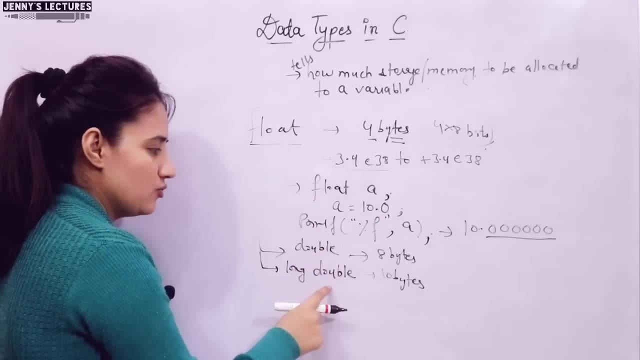 will take 8 bytes to store in memory. if it is long double, it will take 10 bytes to store in memory. right, and the range would be greater than float and the long double range would be greater than this double. But you don't need to remember these ranges because they are very lengthy, right and 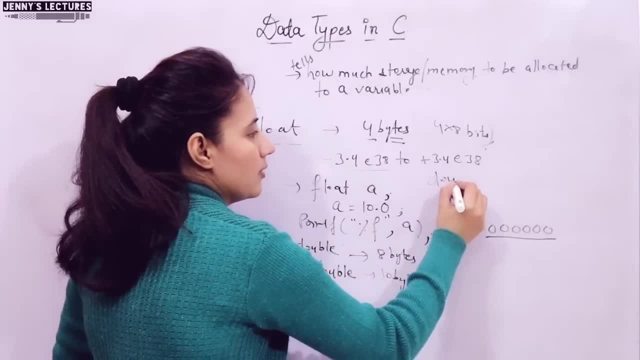 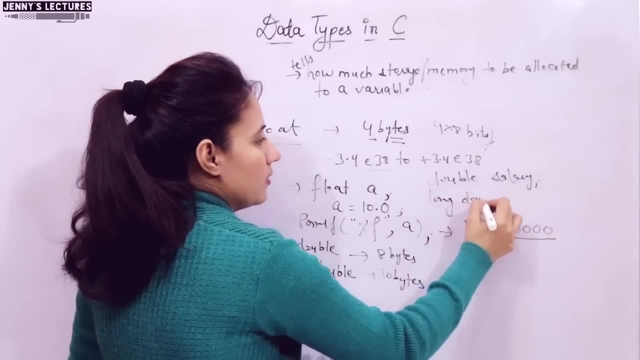 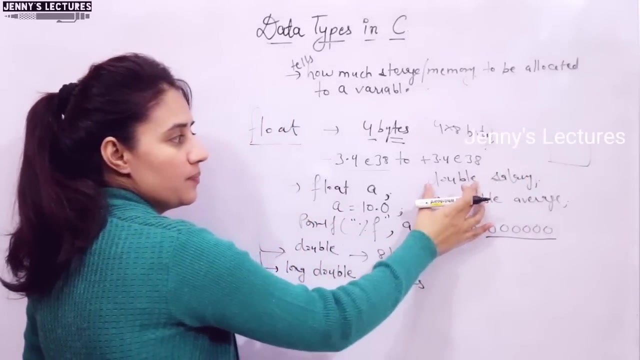 to declare a variable of type double, you will write double. suppose I am writing here salary. if I want to declare long double, you can write down long double now salary. this name in memory space would be allocated. how many bytes? 10 bytes right, and for this average, how? 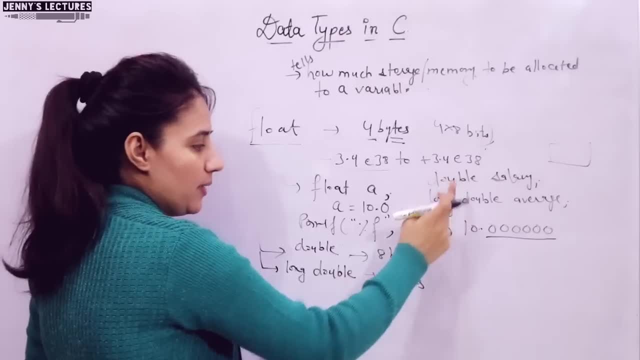 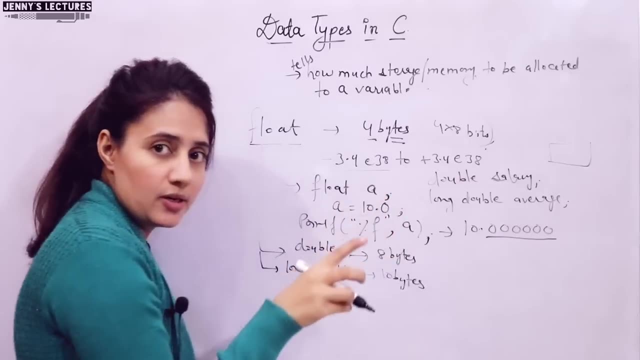 many space would be allocated in memory. 10, sorry, here 8 bytes, Right 10 bytes, and here the space would be allocated for 10 bytes. and, yeah, for double to want. if you want to print a variable or a number that is of type double, then here you will. 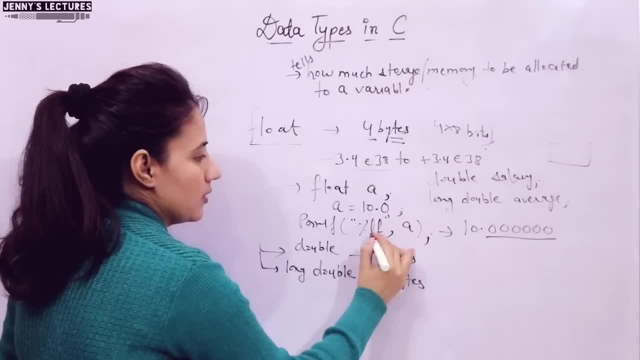 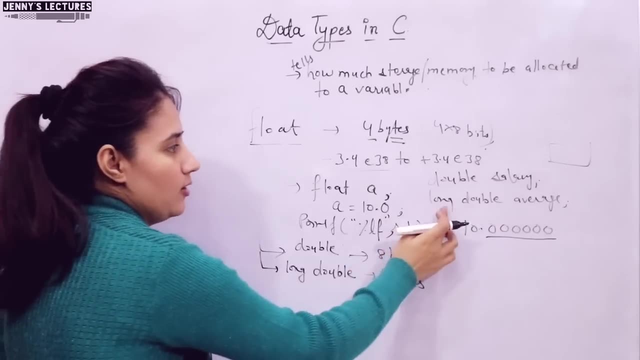 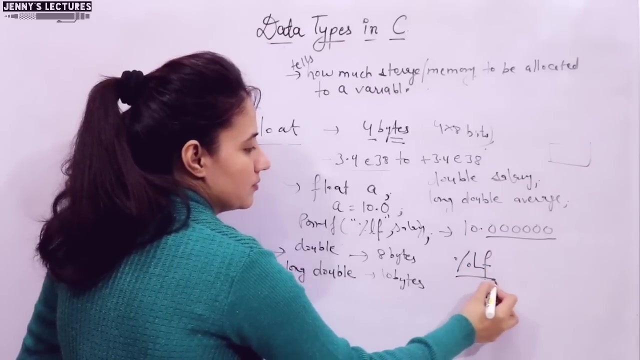 use lf, lf, and here you can write this salary right. and if you want to print a long double number, then what you will use percentage capital, L and f. I am not sure, but you can search it and you can tell me if I am wrong in the comment box. 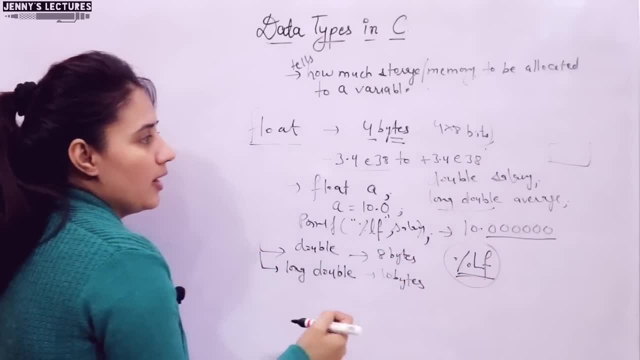 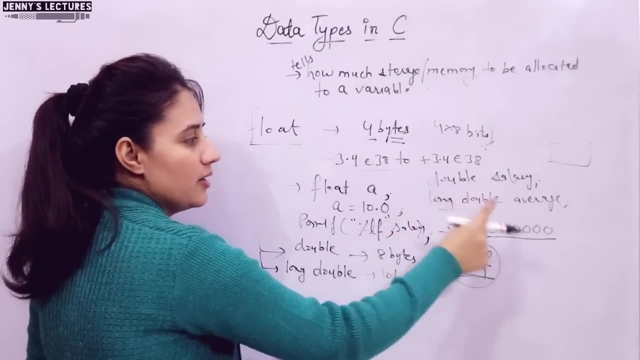 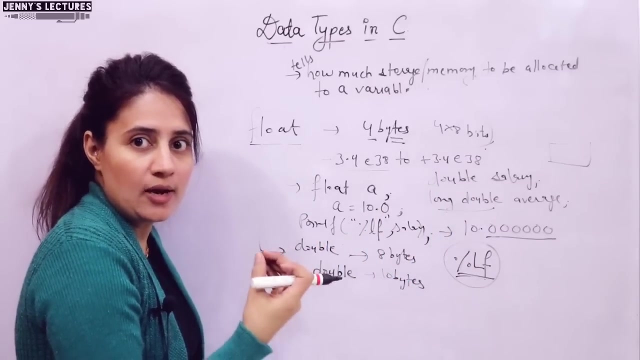 the format specifier for this long double right. and one more difference is what the number of precision after decimal is what? 6 digits in float and in double it's 14 digits. so that number is having more accuracy, right? if you want to perform some calculation, which? 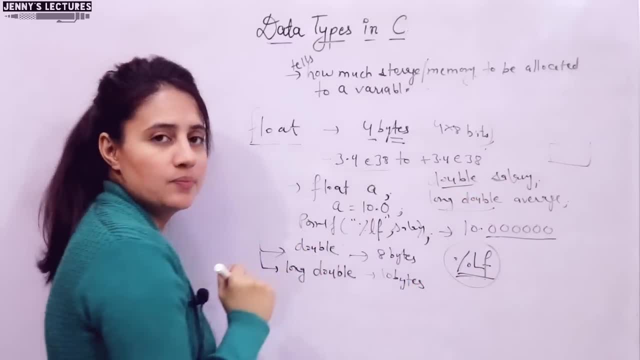 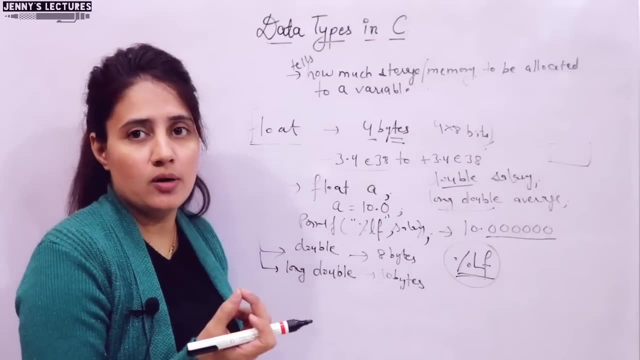 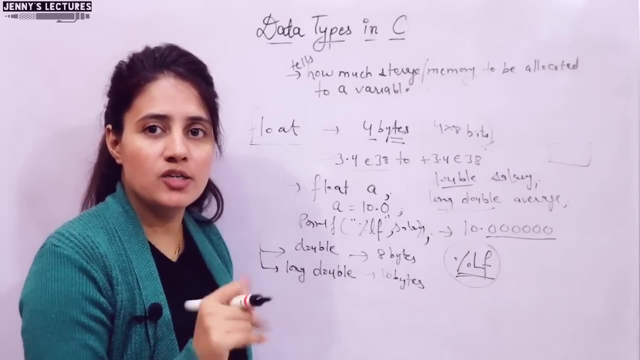 require more accuracy, then we will take this data type right, otherwise we will take float right. So these two types are void data type, but void we don't use to. we don't use with variables. void means empty, nothing is there. so we use generally this data type with functions.